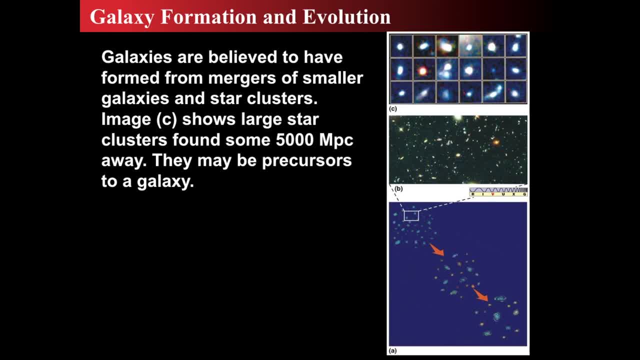 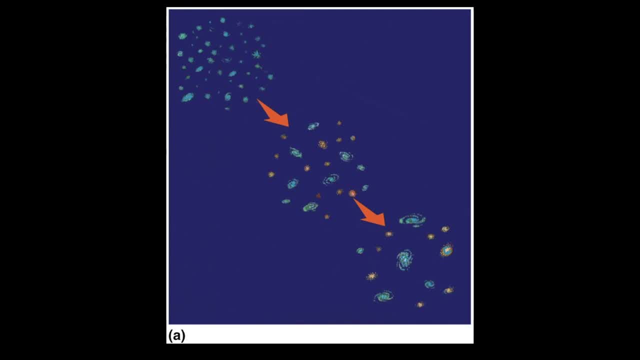 galaxies have evolved with time, and that's really what we're going to be talking about now. So it's thought that galaxies go from small, misshapen, extraordinarily blue objects and go by mergers and mergers and mergers into forming spirals and giant ellipticals. 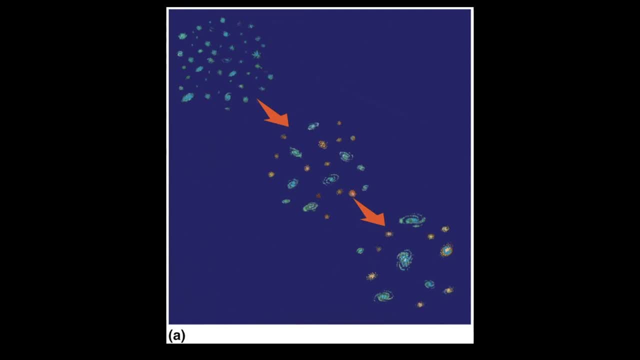 So it's thought that galaxies start in very tiny things and grow through gravity, And that's what we think it is. Now, given that's the concept, we should look for that in the observational evidence to see if this general sketch is true. 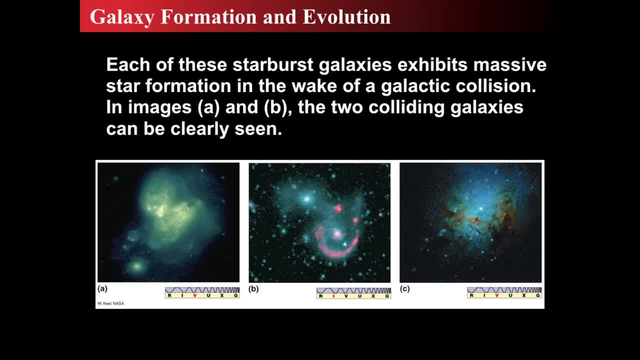 So we can also think that there's definitely evidence for collisions because, as we saw, starburst galaxies have massive star formation. We could actually model the appearance of starburst galaxies by colliding, and the collision, collision models and numerical models that show collisions between spirals can actually 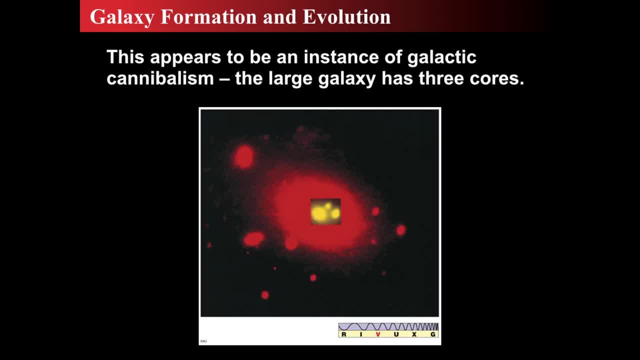 accurately map objects that we see deep in the sky, And in fact, we see some places that look like they have multiple cores, like some galaxies are supermassive, giant elliptical galaxies and appear to have multiple galactic cores, and so they must be in the process of merging. 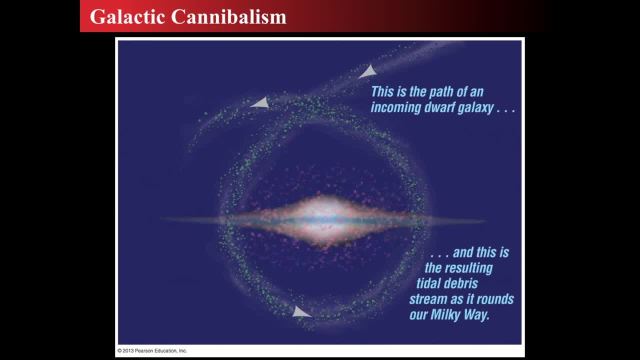 Also we know about stellar streams. There are stellar streams around other galaxies and there's also stellar streams orbiting our Milky Way. and stellar streams are tiny little galaxies that are very low mass, that get spread apart along the line their orbital path and as they orbit they get stretched and pulled and their 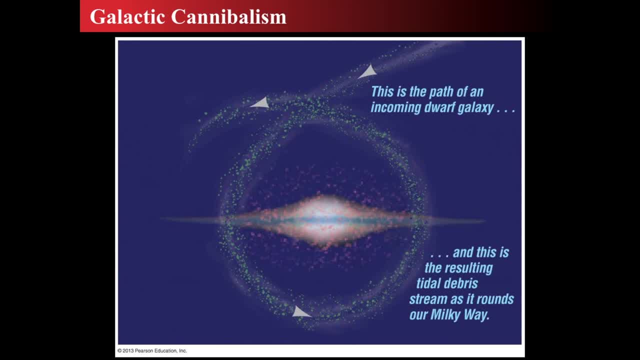 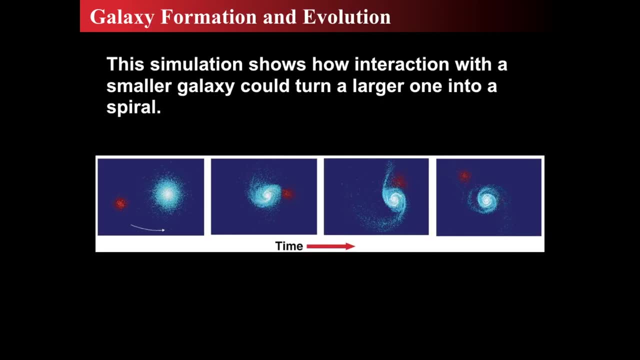 stars get pulled into different orbits and they no longer look like a galaxy but now look like a stream because of the tidal pull between the near and far side of the little galaxy. So we should expect that larger interactions actually will create maybe some spiral interactions, Maybe a small. 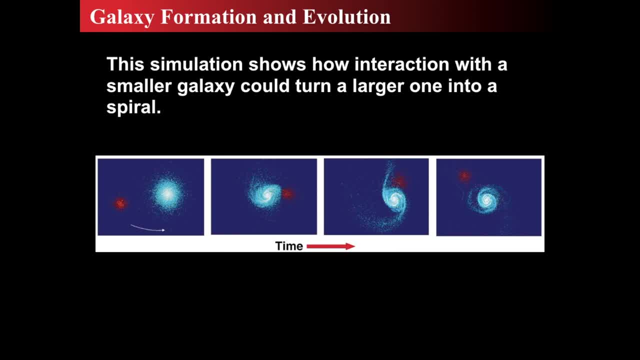 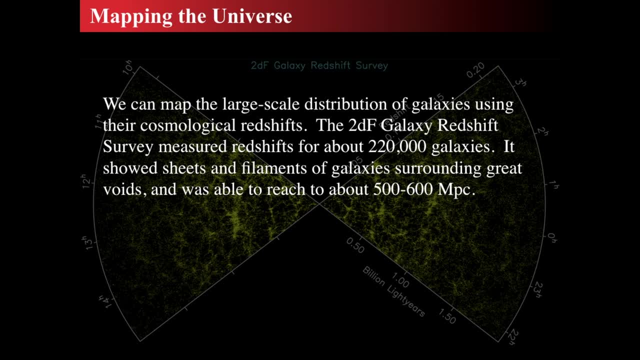 galaxy turn a large one into a spiral. If it still has gas and dust, it spins it up. So we can then say: well, do these evolutionary characteristics actually appear in the data? And so if we look at massive surveys such as the 2DF galaxy redshift surveys looks at about a quarter million galaxies. 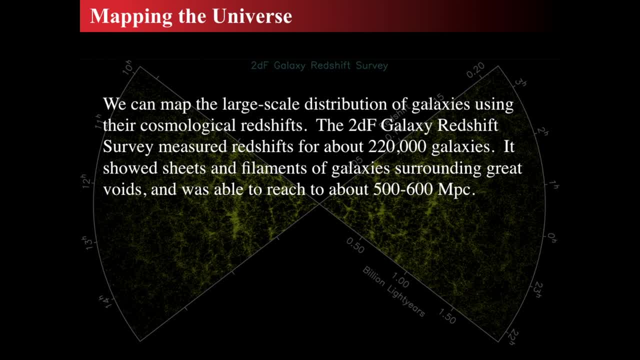 and they showed that. yeah, they're distributed in sheets and filaments and voids, and what's been looked at by this specific survey goes out to about almost two billion light years, and there we'd have a better view of it. 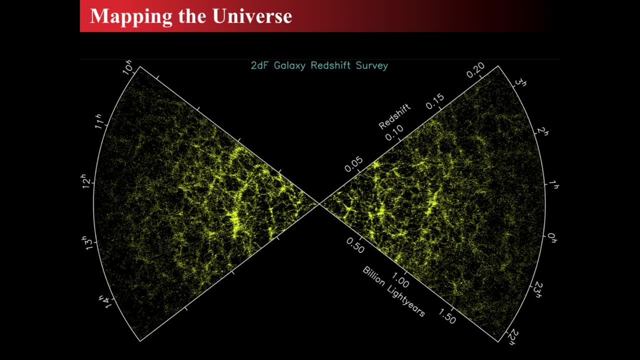 and we see the redshift is about to about 0.25, or about a quarter, and that's a really good way of measuring Instead of billions of light years. redshift is the big thing that we're going to be talking about. 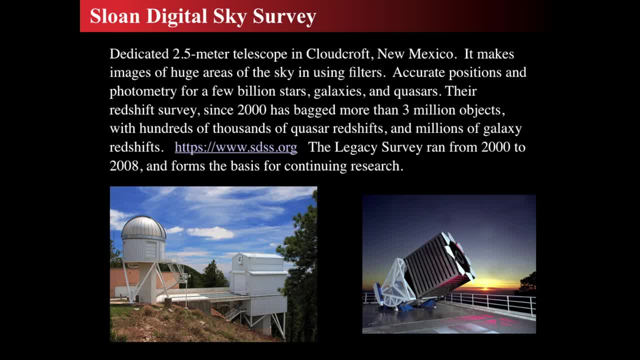 So the other one that's actually been a significant contributor to the universe, our understanding of the universe, is the Sloan Digital Sky Survey, which was a large two and a half meter scope in Cloudcroft, New Mexico, and actually went to grad school in. 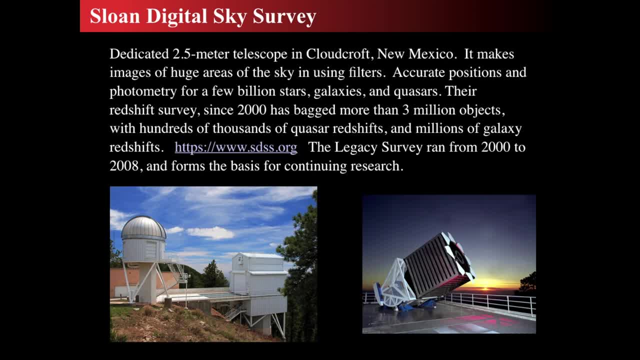 New Mexico State and I started off the very, very, very beginnings of the elements of the computer technology that went into the stuff And so back since the early 1990s we're talking. this is like the beginning of the Internet. So you know, nowadays 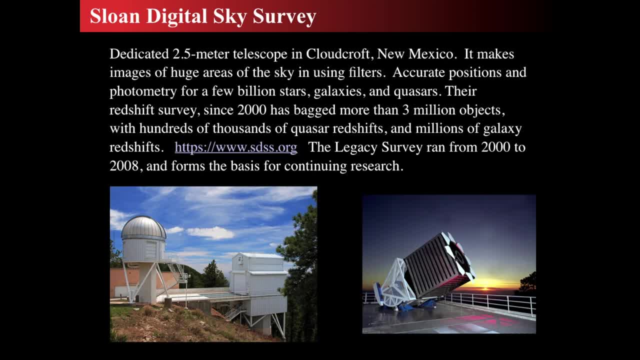 what I did was kind of minor but yet it was groundbreaking in its time And that's helped me to do other things in my life too, which is kind of neat. So this particular telescope, though the Sloan Digital Sky Survey which is demonstrated, which is shown here, 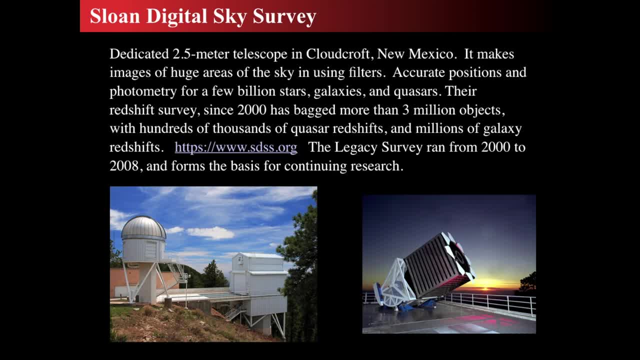 its goal and its major survey ran from 2000 to 2008.. And it cataloged millions upon millions of objects with hundreds of thousands of quasar redshifts and lots and lots of galaxy redshifts, And it got photometry for billions of stars, galaxies and quasars. And the goal with this thing. 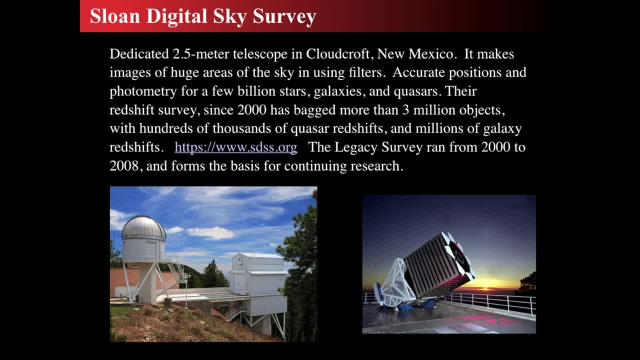 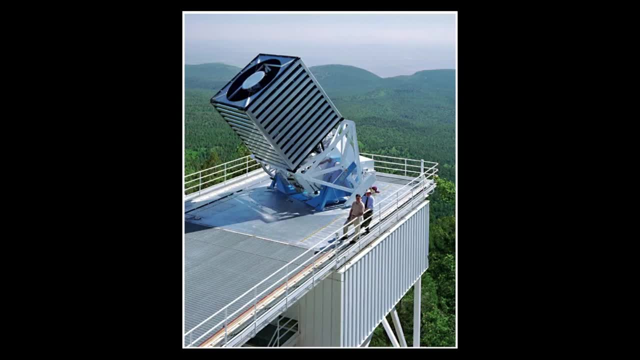 was to make an accurate map of the sky and specifically hunt for galaxies and their redshifts. And there it is, over the Sacramento Mountains, And in the distance you can see the White Sands National Monument. So this is a beautiful place And if you ever get a chance to go to New Mexico and get up to Cloudcroft- 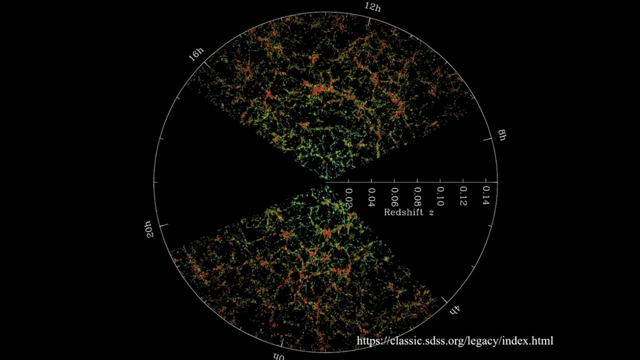 and say: hello, do it. Anyway. this is one of their data sets. This comes out from the Sloan Digital Sky Survey. This comes from what they call their classic legacy archive, And it shows out to a redshift about 0.15, which is: 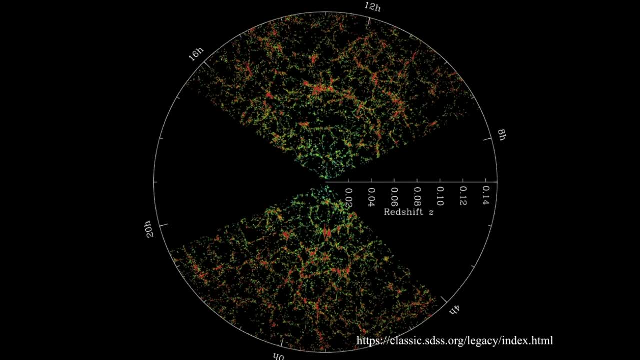 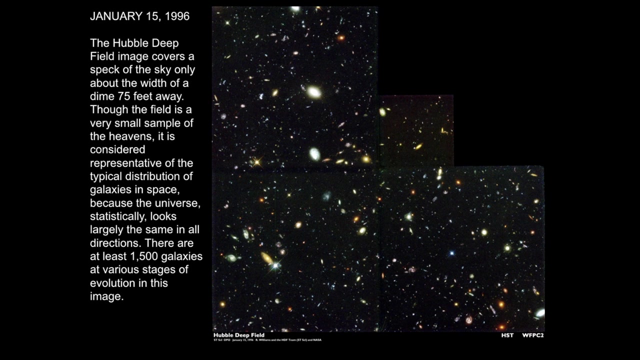 not as deep in this particular image as the 2DF survey, But over time the Sloan Digital Sky Survey went much deeper and had many and much larger data set than 2DF. Well, can we find that takes a little bit, So let's go back a little bit further and see why the Sloan Digital Sky 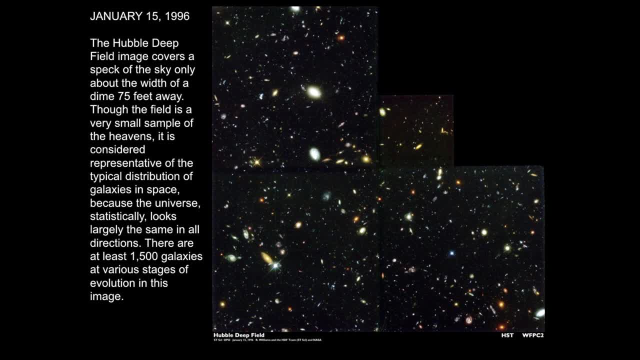 Survey was even done and why 2DF was done, and what motivated people to make these massive surveys. Well, the Hubble Space Telescope was launched a while back, and one of its major goals was to actually study the evolution of the universe, And what this was was the longest at the time. 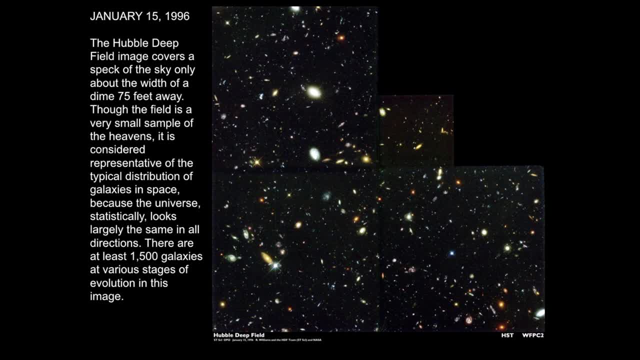 it was released in January of 96.. It was the deepest survey yet done by any telescope ever, And so this is what we call a pencil beam survey, And the Hubble Deep Field allowed us to see galaxies back to about 13,- almost 13 billion light years in distance, But we see that there's all. 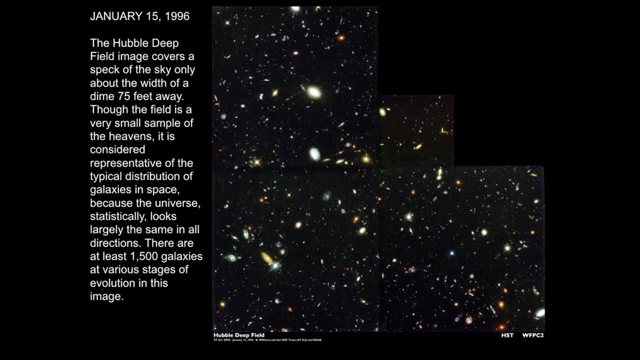 sorts of arrangements and appearances to galaxies. There are about 1,500 galaxies in this image alone, But remember that the size of this image is very tiny. It looks kind of big here, But if you take a dime and put it, 75. 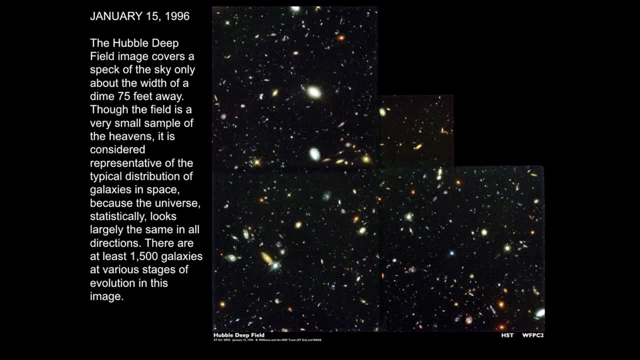 feet away. that is the size of this image in the sky. So it's a very, very, very, very tiny image of the sky, And if 1,500 galaxies are in this direction of the sky, then they're everywhere, And then 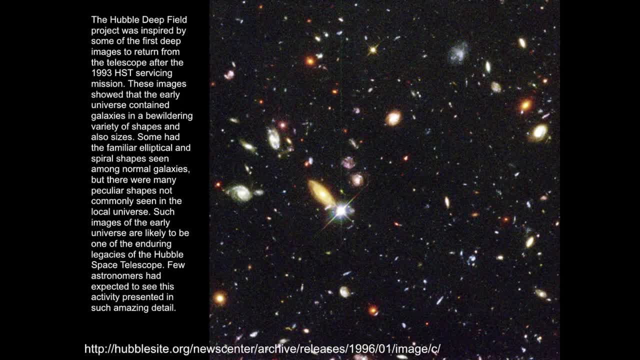 this is not the deepest of the surveys, But this was the first one And here's some elements from it, And the details were pretty controversial when it first was done because nobody actually thought that this would actually use Hubble time wisely, But it ended up being an amazing, amazing set of discoveries. 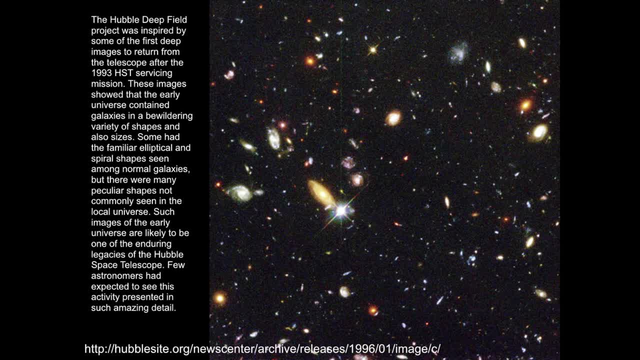 And we see. most of the objects in here are galaxies. There are some faint red dwarfs that are Milky Way objects. Those would be the stellar objects that are in the foreground, But most of the tiny, tiny, tiny objects in the background are galaxies. 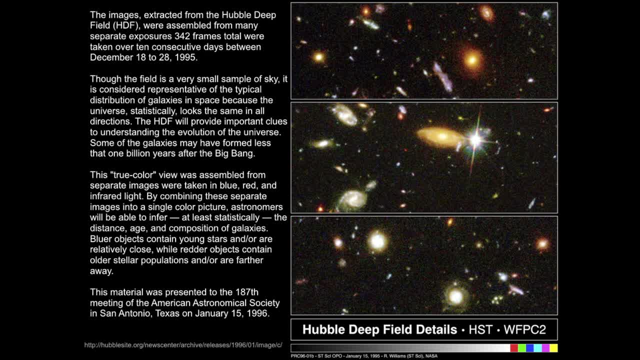 Again. here are some more details from the Hubble Deep Field And there were 342 frames taken over the course of 10 days, So this is a huge, huge undertaking, And the size of the area was this was one of the longest exposures ever done to date. 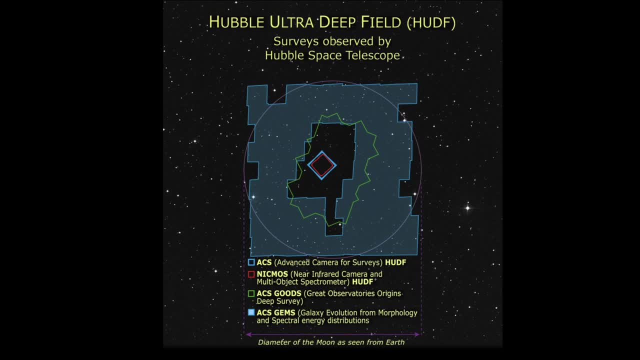 in 1997.. All right So, but that wasn't the first. then, Considering that that was something that actually yielded results, then people said, well, let's keep going, Let's keep going and get more. So the Hubble Ultra Deep Field based in part on that. 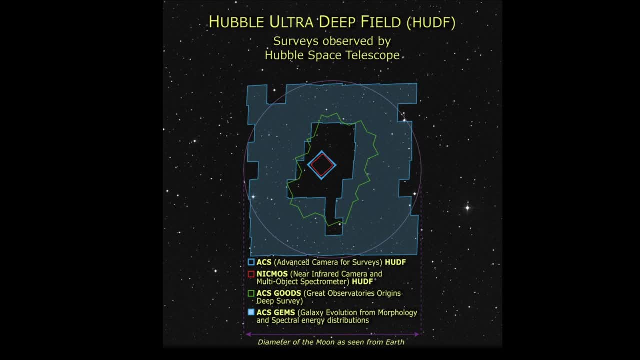 surrounding that area. And so what you see is that the purple circle here shows what the Hubble Ultra Deep Field looked at, And that the circle illustrates the size of the Moon. And then there is the green outline, which is the Goods Survey, And this is 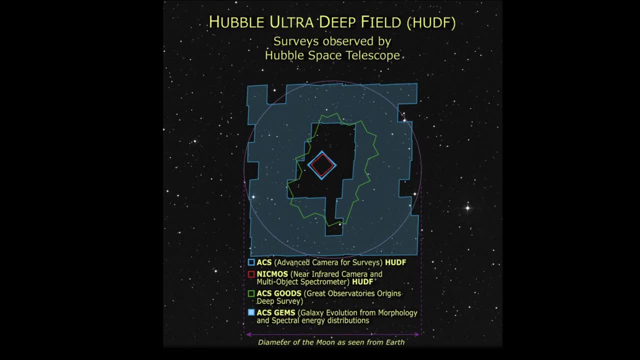 the Goods North group, And so there's a very large image that was created out of that, And the Advanced Camera for Surveys on the Hubble Space Telescope is a tiny little blue block in the center, And the Near Infrared Camera and Multi Object Spectrometer or NICMAS, also on. 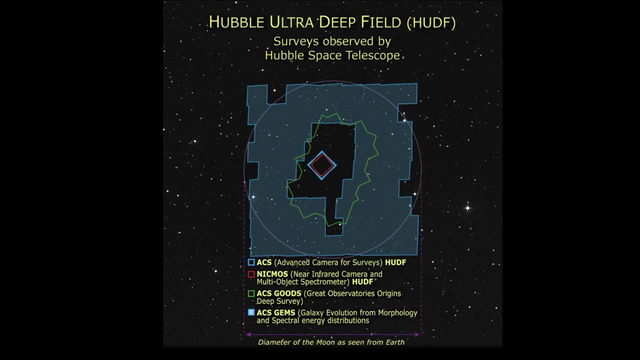 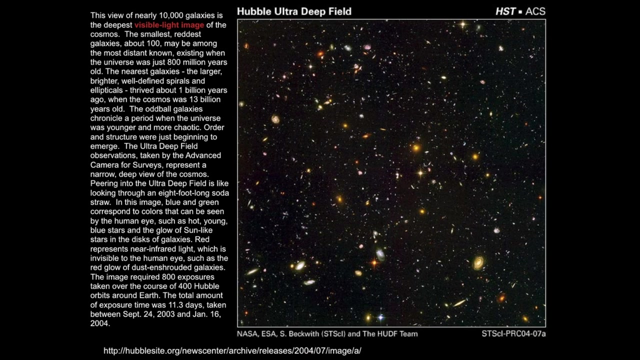 the Hubble Space Telescope was used to do deep imaging, So a series of images were given in this whole area in order to discover exactly how deep, what kind of depth we had, And the Hubble Ultra Deep Field then was released in 2003.. And 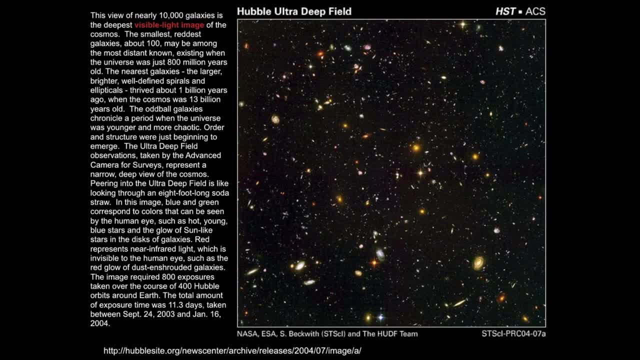 that's about six years later, And this holds some of the. this also contains the Hubble Deep Field, But it is a there's now 10,000 galaxies in this visible light image, And so they used a large, so now the visible light. 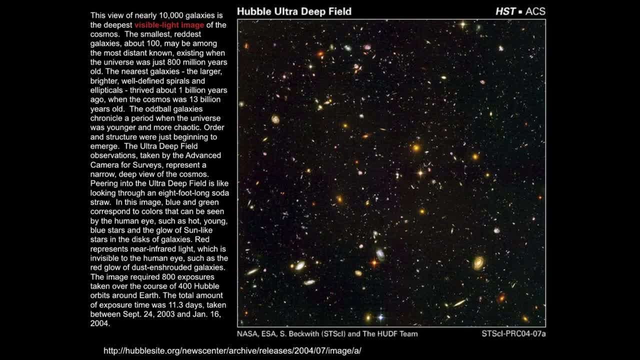 band was used And there are some very, very, very red galaxies And the dimmest objects and tiniest galaxies were when the universe was only about 800 million years old. And so, as you see through, when close ups of this image show that when the when you look at deep, deep, deep, 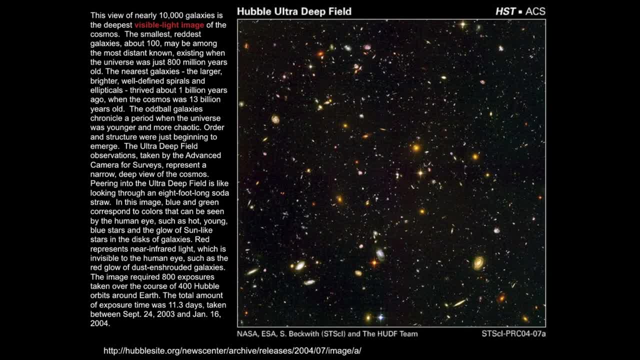 into this image and look at the highest redshift objects, then those are small, blue, misshapen galaxies And you only get fine structures like spiral galaxies in the local universe, meaning today, And with this, there's something really interesting about this that we'll get to, But this again was 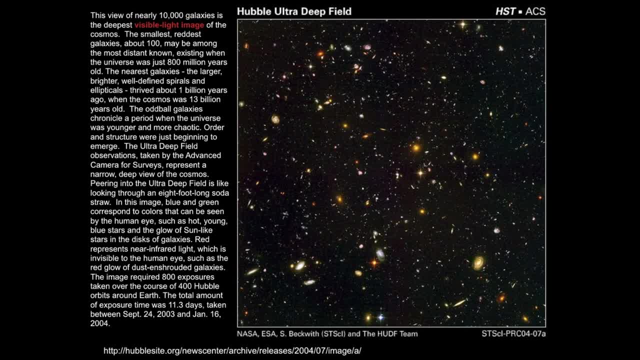 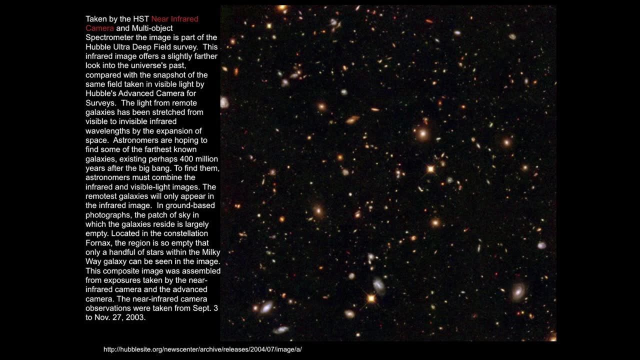 an enormous undertaking with 800 exposures taken over 400 orbits of the Hubble Space Telescope around the Earth. about 11 days of exposures And this utilized the advanced camera for surveys. And then they utilized looking at with the NICMAS experiment, looking at the near infrared to actually look at objects. 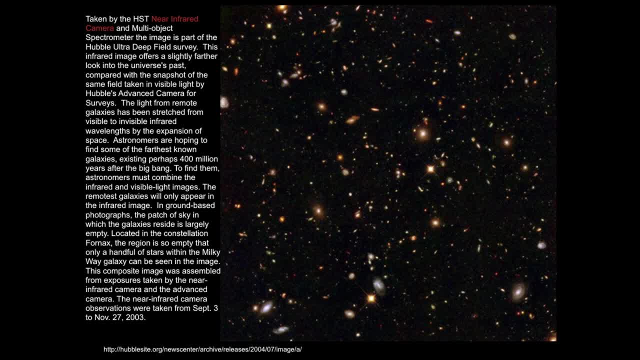 who would be strongly redshifted, And this gives an important element to see what are the deepest objects in this field. And that allows you to see further back in the past, Because if something is getting greatly redshifted, it will probably appear in the infrared. 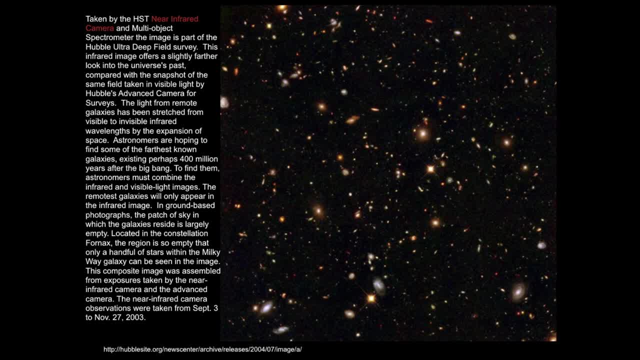 Rather than visible, And so you can actually see farther back in time using this, And that's why we see that this, the caption of this comes, shows that it's about 400 million years after the Big Bang would be the deepest and faintest objects inside of. 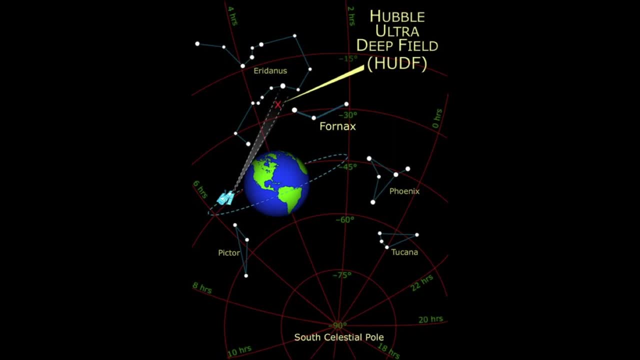 this. So the Hubble Ultra Deep Field is actually in the northern constellations. I actually noticed that this is a southern. this is the Hubble Ultra Deep Field south. It looks in the exact opposite direction And we're looking in the area of Eridanus and the 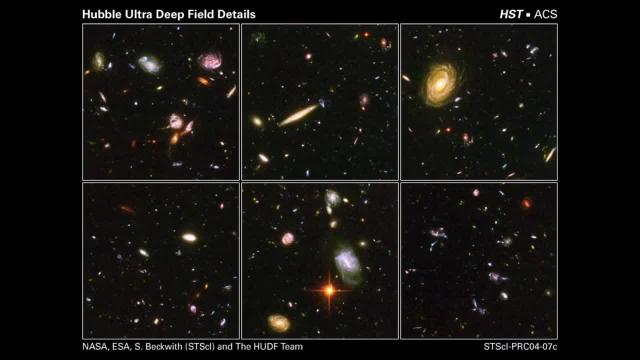 constellation Fornax. So there are many details in the Hubble Ultra Deep Field that show the evolution and state of galaxies. You can see some extraordinarily misshapen objects And only the larger objects meaning the closer objects, meaning objects that are in the local universe, are actually things that are. 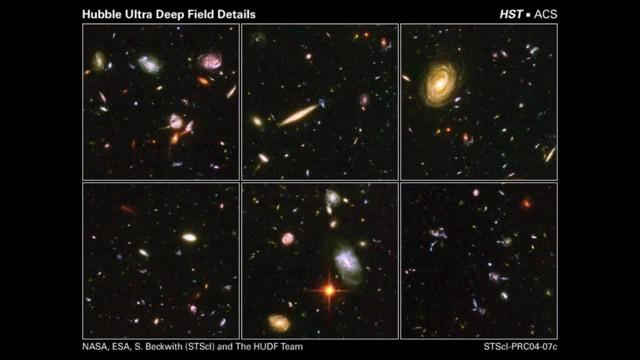 grandly structured, such as spiral galaxies, But if you look in, say, the lower right image of these sects, you see in the upper, in the kind of the right, left hand side of the upper lower right object, you see a really distorted and misshapen thing. In fact, all the objects 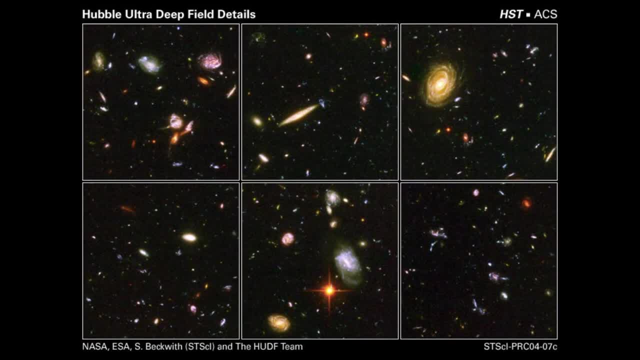 in there are distorted and misshapen, And only recent objects, meaning very nearby and at low redshift, have the appearance, And what we're actually beginning to see is that the something that looks like the Milky Way only appears now. If the universe had was infinitely. 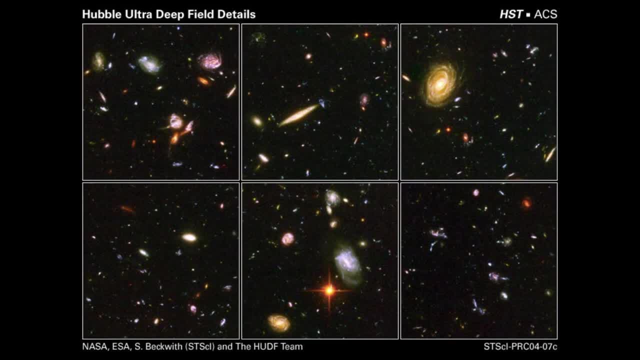 old, then we should expect to see things just like the Milky Way, But extraordinarily far away. We do not see that. What we do see, though, is the Milky Way is only a recent thing, And if we look farther out into space, and therefore farther back in time, we see that there is. 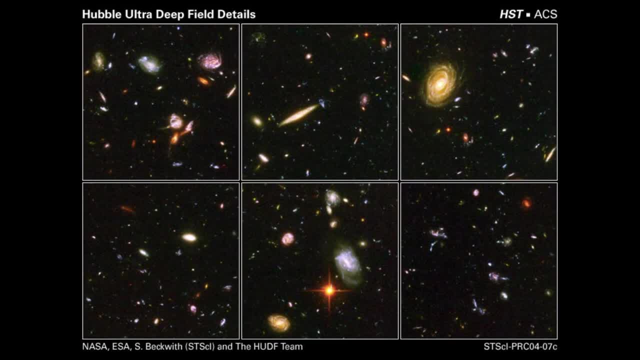 an evolution of galaxies from then to now, And we do not see anything in the deep, deep, deep past that looks like anything like the Milky Way. So this is again a prediction of the Big Bang: that there would be a baby picture of the 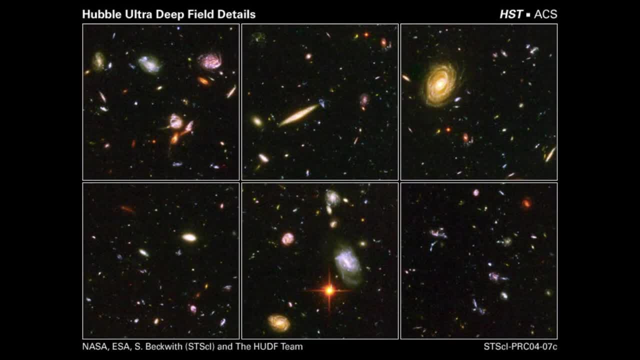 universe and an adult picture And baby pictures predict that if the universe had a beginning, then if you look farther out into space, you're looking farther back into time And therefore you should see things as they were ago. And if the universe was infinitely old and didn't have a birthday, then you should see Milky Ways. 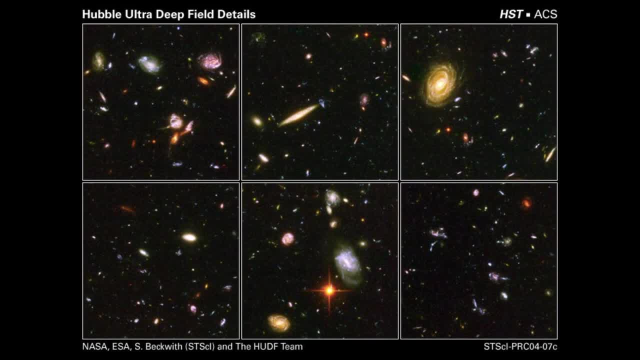 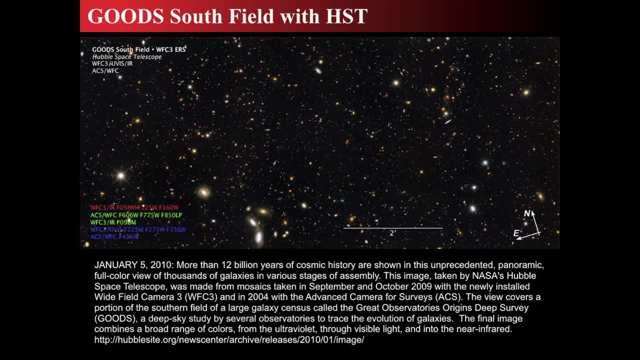 and things mixed in with baby galaxies, But we do not see that. We only see baby galaxies long ago and far away. So the Goodfield South that we described a bit, this was presented at the AAS conference- American Astronomical Society conference- in January 2010.. 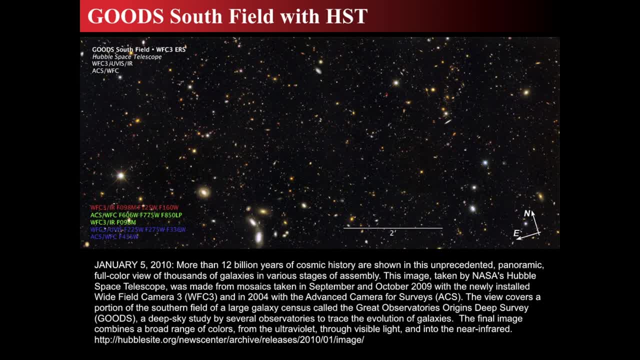 I had an interesting time seeing this. They printed this out and put it on a wall at high, high resolution. It was about 30 feet long, I think, and about 15 feet high. It was an enormous, enormous poster that they printed out. But the goal with this thing was again to show that the 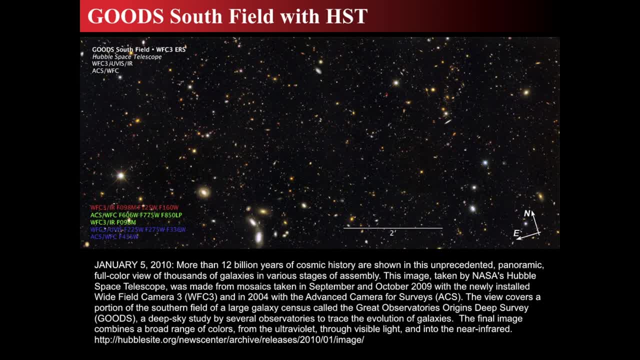 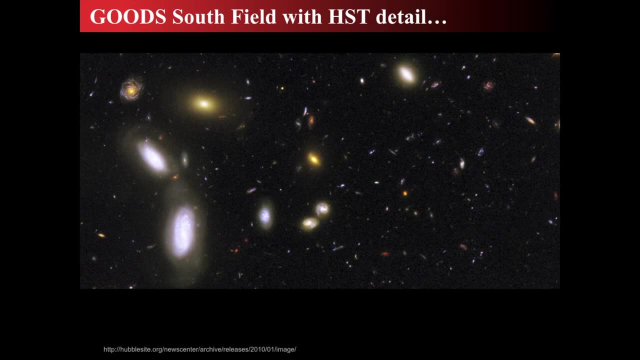 images of galaxies could be seen when we look perpendicularly to the plane of the Milky Way, And as we look very, very far, deep, deep out, we get to see how galaxies have evolved with time, And here are some details from that image set. As we zoom in, we see many, many galaxies, But the deepest. 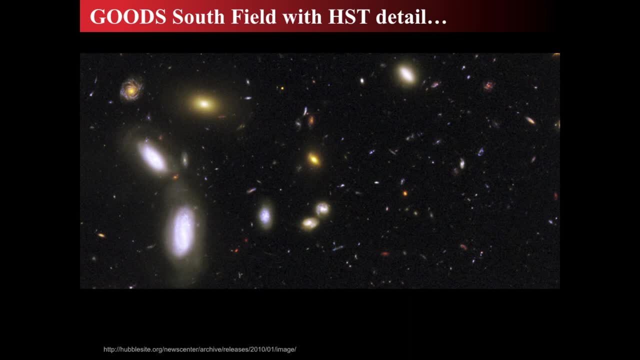 tiniest, even the tiny little flecks, those are galaxies. Those are because they're misshapen and they don't look like point sources such as stars. Now, there are a few Milky Way stars in this image- quite a few, But most of them are, but there's most of them. 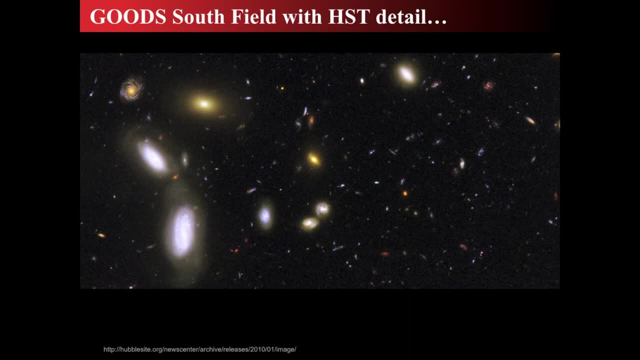 more galaxies than stars. So the fuzzy objects are galaxies, And on the left hand side we see a number of tiny galaxies or globular clusters or dwarf kinds that are being that are interacting with the two near spirals that we see. 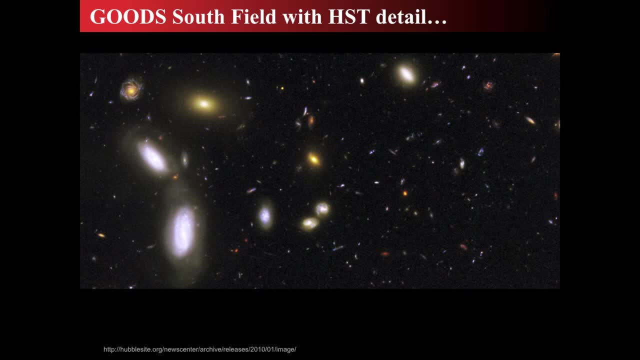 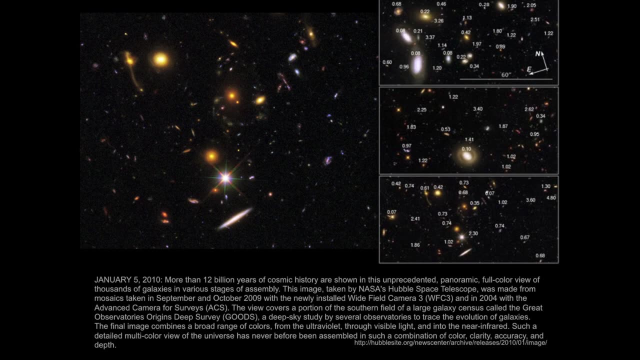 And we see kind of a little spiral off to the upper left that is much further away, And here's some details inside of that as well. We see kind of a cluster and some gravitational lensing effects on the upper left. there We see a gravitational lens to the galaxy And 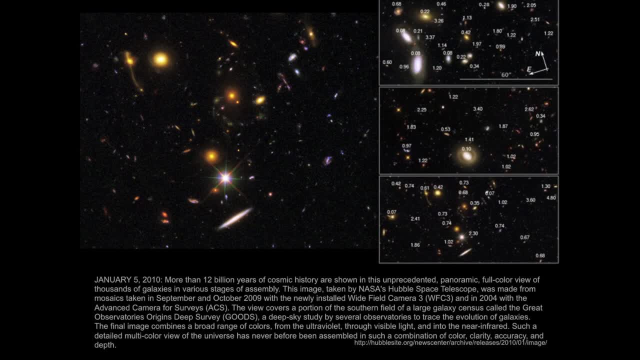 we see the ranges of redshifts in here. so, if you can go, i will post the actual the the actual images and the location where you can find this on nasa's website so you can go, take a peruse, so you can see how far back in time we look. all right, these are some really cool images. 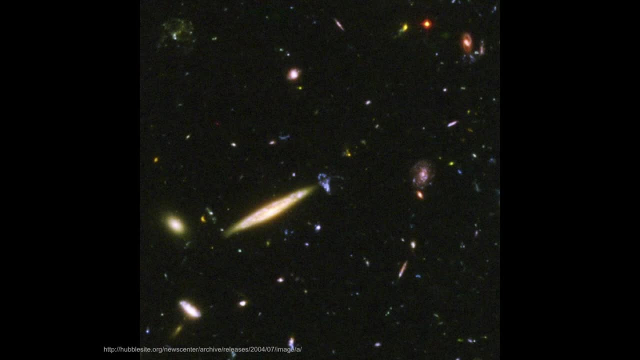 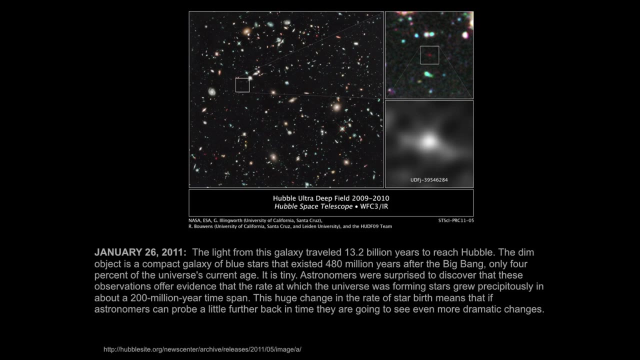 and again, almost all of the things that we see in this image are galaxies as opposed to as opposed to stars, but part of the ultra deep field that was observed were some extraordinarily high redshift objects. so in 2011, a particular ultra, ultra, ultra distant object was seen. 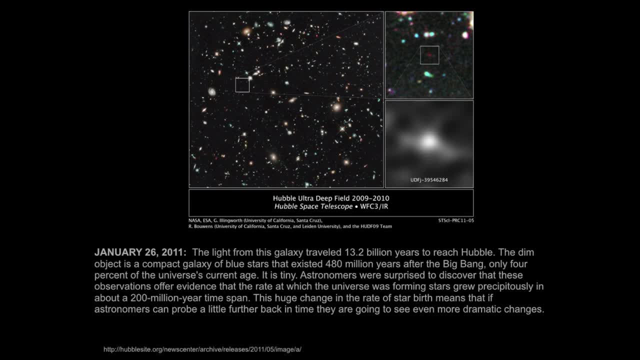 where its redshift was measured in a very special way, which i'll describe in just a bit. and if it is a tiny, dim, misshapen compact galaxy, you've just made up of blue stars. wait a second. if it's made of blue stars, why would it be red in the image? uh, well, okay, since. 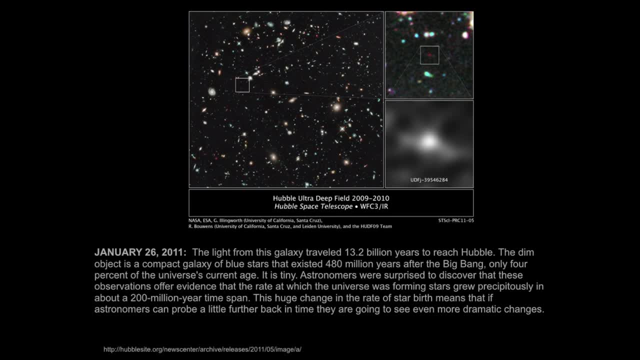 it's not like a mystery game. it's red because it's been redshifted. it's been redshifted deep into the infrared. but the in order for it to be seen deep in the infrared, it must be extraordinarily bright and if there, and if it's high, high, high redshift and still visible in the 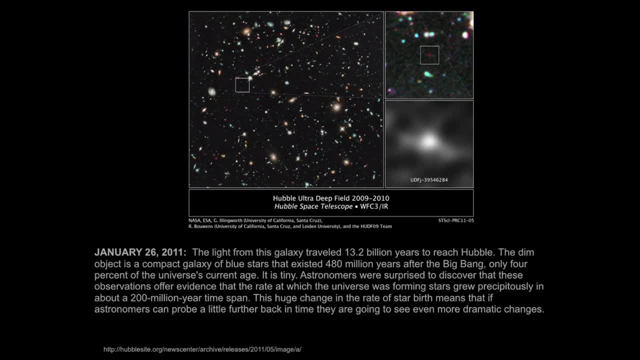 infrared, then therefore it must be bright and therefore these whatever was emitting, it was emitting copious amounts of blue light. so this is a time when this particular galaxy, whatever it looked like, was a mishmash of stellar activity. so let's zoom in and take a look at what this ultra. 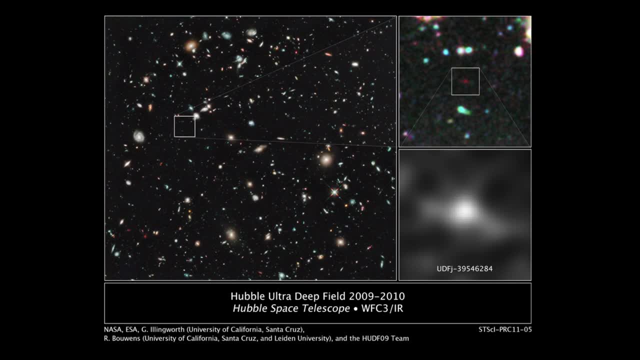 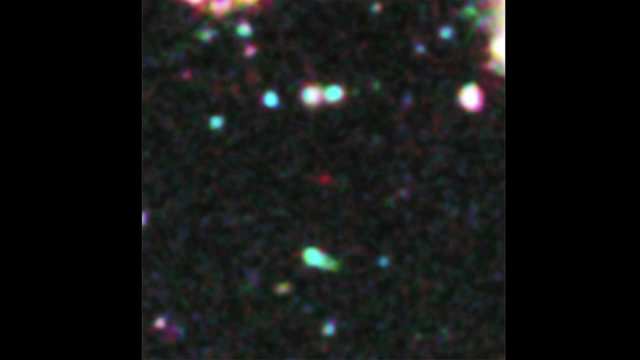 deep field object is, and has the highly enjoyable name of ultra deep field j39546284. okay, that's not very illuminating. uh, this was done by illingsworth at santa cruz and bowens and hubble, ultra deep field 2019, and so we can zoom in and see this little bitty, tiny red dot, which is this ultra. 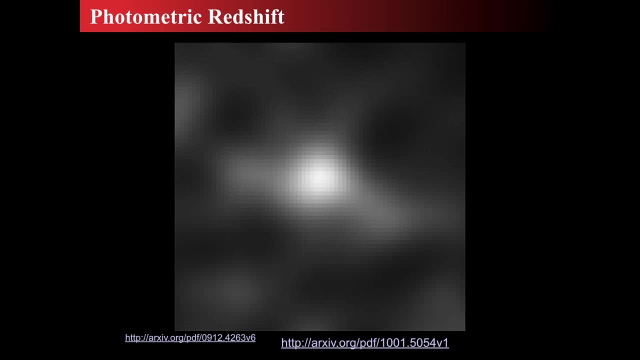 red, high redshift object. and well, you know, now we're looking at the actual pixels on board the hubble space telescope itself and that is the, the pixelation that that blocky appearance is the appearance of the actual object in the picture itself and the boxes. 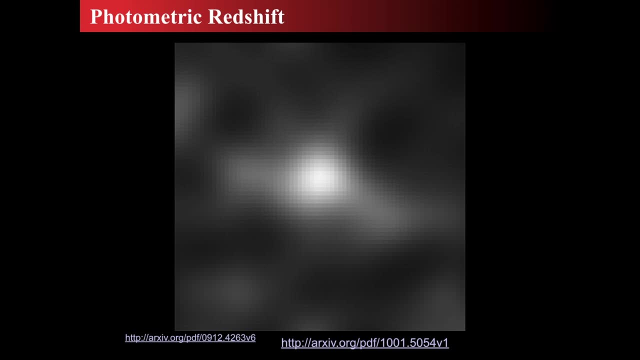 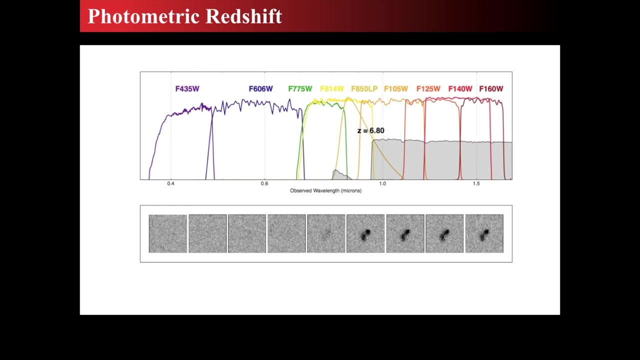 are the individual pixels on the camera for the for the hubble space telescope, and i provide a couple of links here that show an interesting thing we're going to talk about called photometric redshift. so photometric redshift is what you can do when you have a high redshift object and a lot. 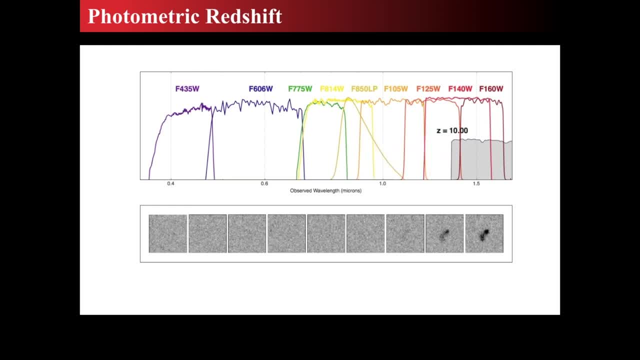 of filters. so the hubble space telescope is outfitted with a huge number of of filters that it can use to put in front of of the camera. so what they'll do is they'll focus on an object and then they'll take an image of it with one filter, then another, then another than 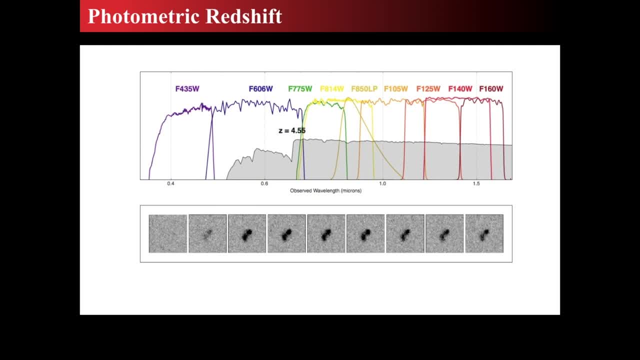 another. and if you steady on it and look at now, we've got this funny thing going back and forth. okay, so what we're seeing is an image of a galaxy, and if it's red, shifted, it will simply disappear from the long wave, the, the short wavelength, meaning the permanent. 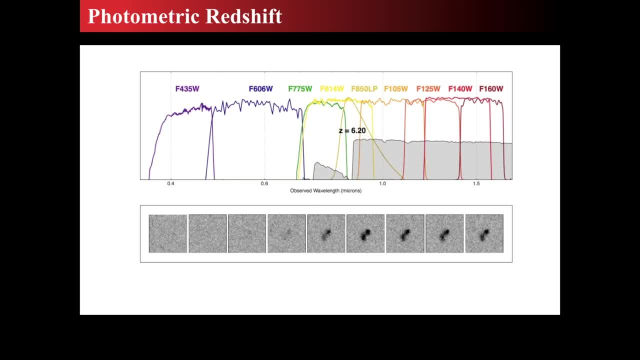 wavelength of the galaxy is the purple and blue side of this, which would be the left hand side, and as it's getting redshifted, it will be appear only on the right. so why does the light disappear and go to zero? that's because there's hydrogen gas in the way and as the light traverses the 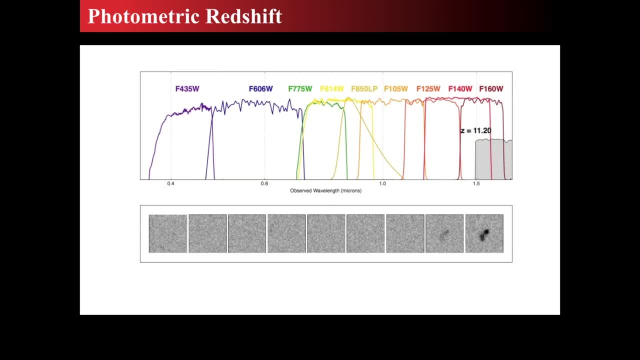 distance of the cosmos as it traverses it. the hydrogen gas absorbs it at a specific frequency, but it's been redshifted so it gets absorbed at every wavelength. uh in between. so there is no light left over at visible wavelengths because as it travels it keeps passing through. 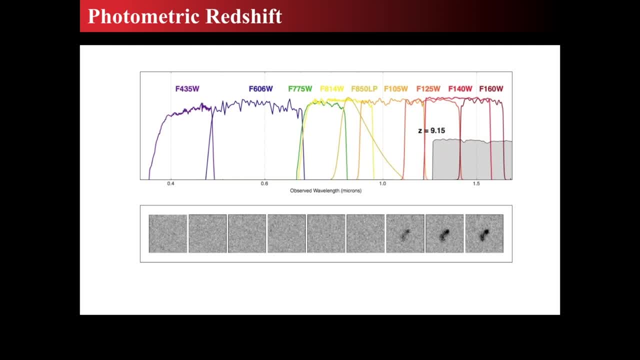 hydrogen gas at different redshifts so it can absorb at different wavelengths. that's really interesting. so we're left with- if you only see it in, the longest possible wavelength filter, wavelength band filter, and that's the only signal- is in the. the long wavelength filters such 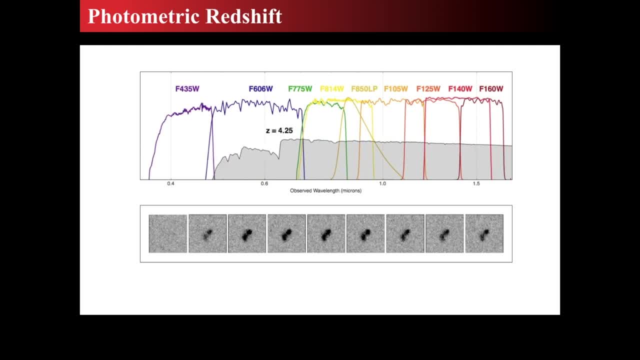 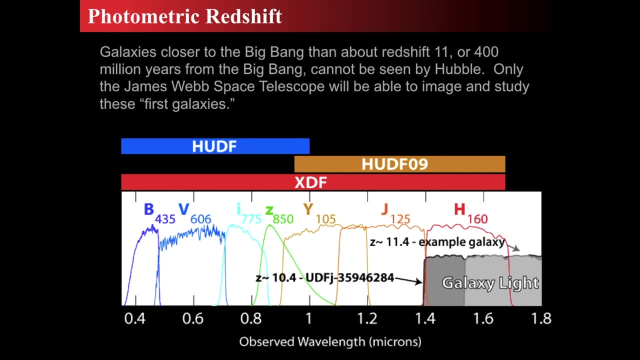 as the f160w that we see there way off on the right hand side, and it's only visible in that one side, one. that means it's been so strongly redshifted that the only way that galaxy can be seen is if it's a redshift exceeding that of 10 or 11.. all right, so an example: galaxy, then the hubble. 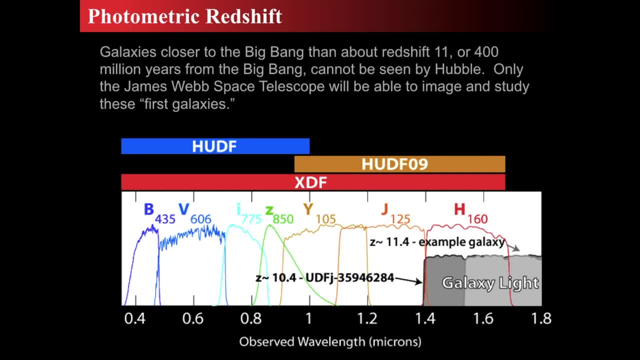 ultra deep field, the hubble ultra deep field 2009 and the extreme hubble deep field, which is xdf, actually integrated all these things together and looked at all the various filters that the hubble space telescope can see. stack them together and found that three, nine, five, four, six, two, eight. 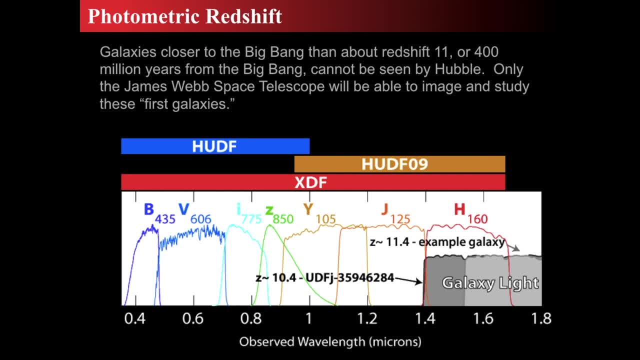 four ultra deep field j object has an ex, has a z or a redshift of about 10, because it only appears in the hubble h filter. it doesn't appear in bv, i, z, y or j filters, and so we call this a photometric redshift, because it doesn't. the galaxy's light only appears at that wavelength, so we think it's. 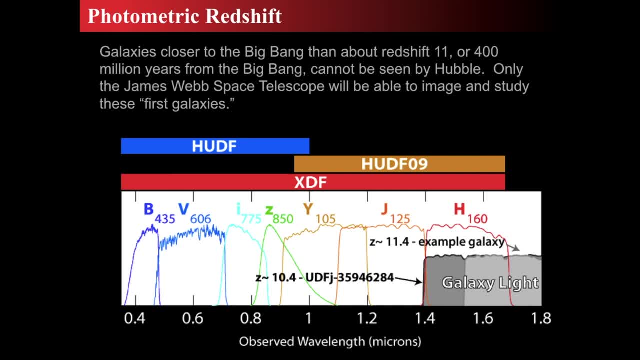 a galaxy and not a foreground star, because a star will still have some emission at a little bit broader wavelength, so it will not. it won't be only at these wavelengths, although it could mirror that. but then you look at the shape of the object, say, oh, it's in this shape and it doesn't have a 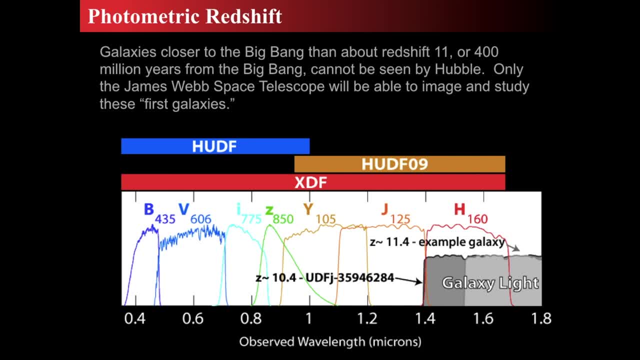 point-like source. so therefore it's probably not a star or some rogue planet in between the galaxies, because those things would be pretty dim, and so the galaxy itself can be observed, and we can posit that because it only appears in one of the filters. it must be an extraordinarily high redshift, and 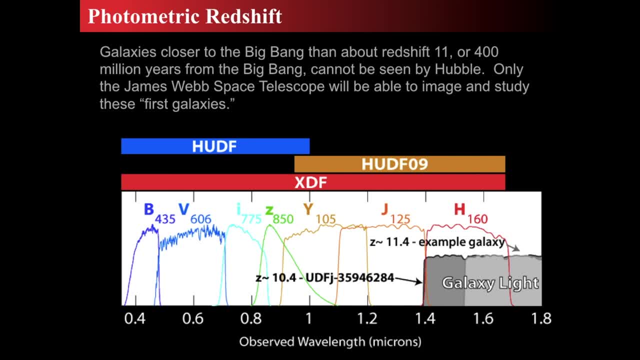 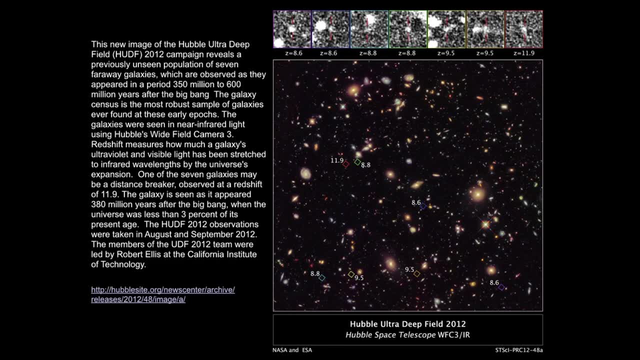 therefore, it set a record of being a redshift of 10, when the universe was 10 times smaller- more like 11 times smaller actually. so the hubble ultra deep field, uh was, was then concluded in 2012, and those observations were taken between august and september, and that included numerous. 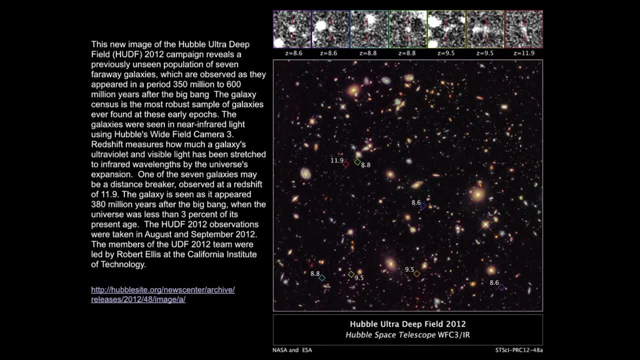 observations. on top of it all, i and using the wide field camera 3 with numbers of different filters, so they actually started adding different filters together and the goal would be then to say: if you can add all these filters up, you can finally get photometric redshifts. and that's what's been highly 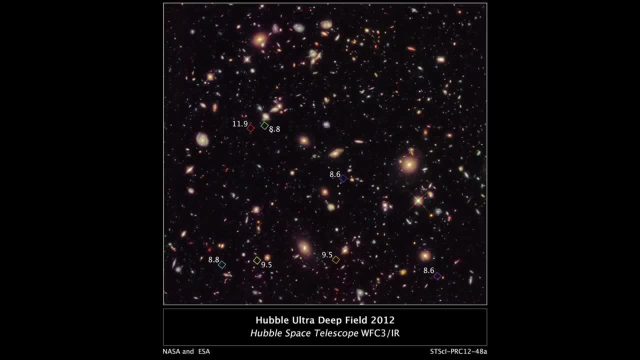 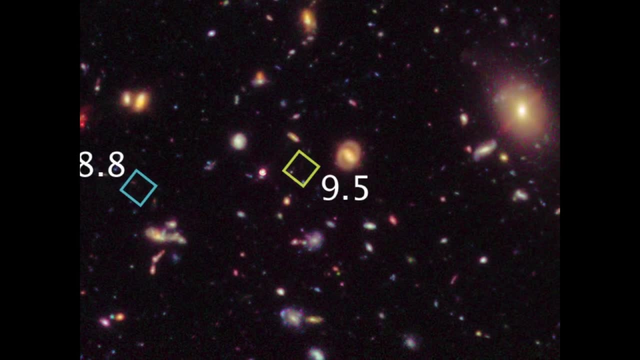 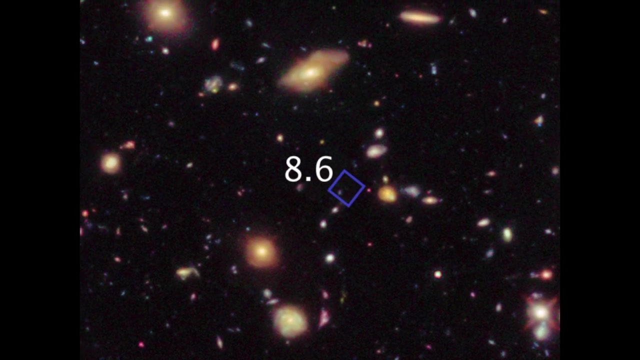 lighted in this image is the highest redshift objects in the entire and the entire field and we see that there's a couple of them at high redshift 8, another one at 10 inside this field, another tiny object at redshift nine and a half and another high redshift object at eight, at almost. 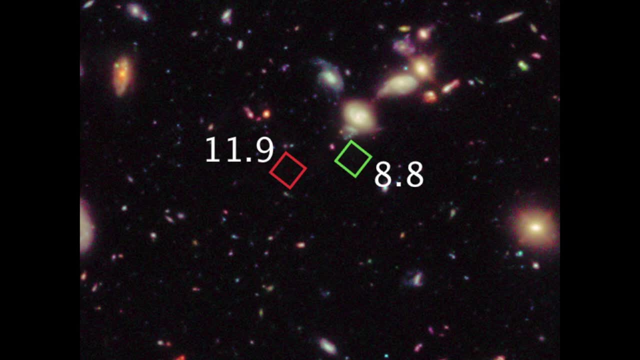 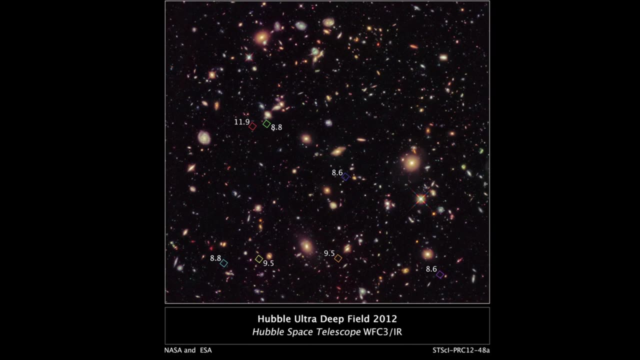 nine-ish. and then the highest redshift object is the one we were talking about at 11.9, which is an enormous time, which is when the universe was 10, was one tenth of its current age, or one twelfth of its current age and 10 times smaller. remember we talked about? redshift indicates the. 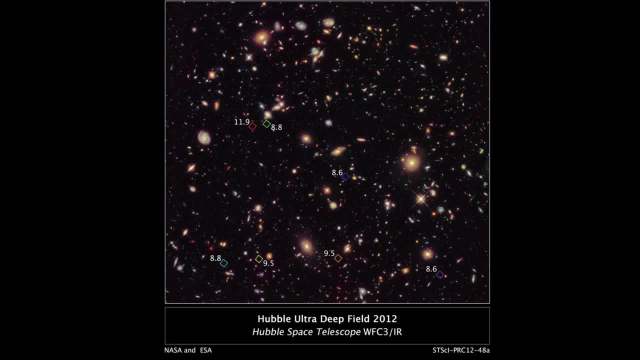 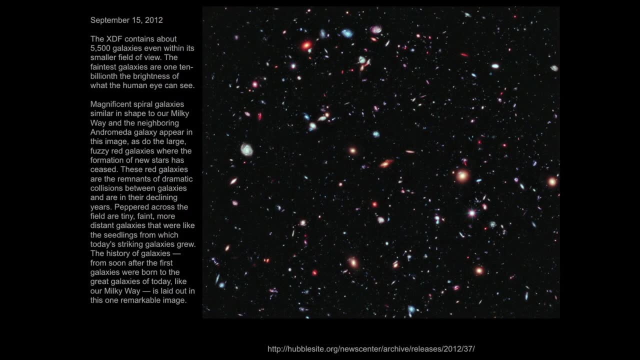 size of the cosmos, so it's actually about 12 times physically smaller at that time. so the extreme deep field then stacked all of these images together and made it for an amazing, amazing panorama. they just- they- took all the legacy data and all their own current data and 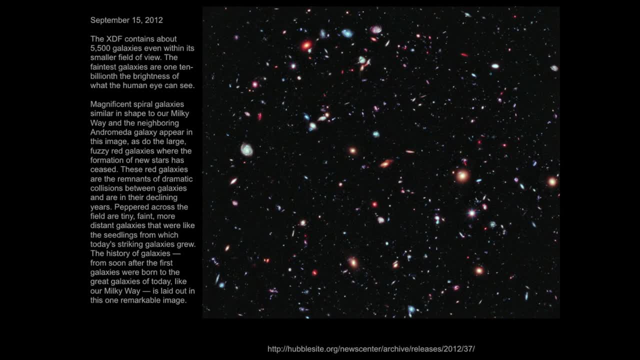 pulled it together to make one image, so it actually had approximately many months of time. this was. this is a common technique that amateur astronomers use in order to stack images together to make a very pretty picture, and it actually cleans up the image, because you can actually eliminate noise by doing that. so the more data you have, the cleaner your data is, and you can say, oh, 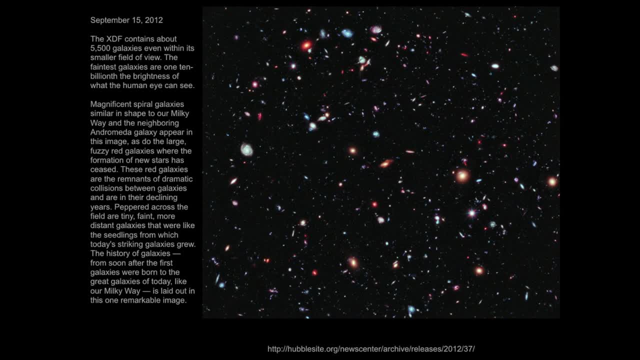 you have a pixel in this image but not in that image, and so that must be its noise, and so this allows the image to be very well cleaned, and the only thing that's left is data. so this one small picture shows the amount of redshift that was produced, that was produced by the supernova. 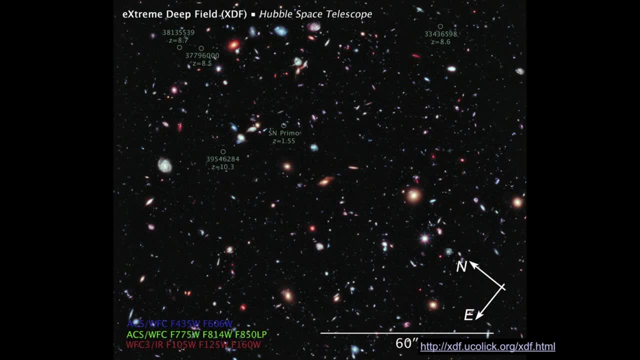 and so i'm going to go ahead and show you a picture of that, and i'm going to show you the, the. the picture that you can see here is the, the image that was taken at a very high speed, and it's the image that shows 5 500 galaxies at various states in evolution, and we see there's the. 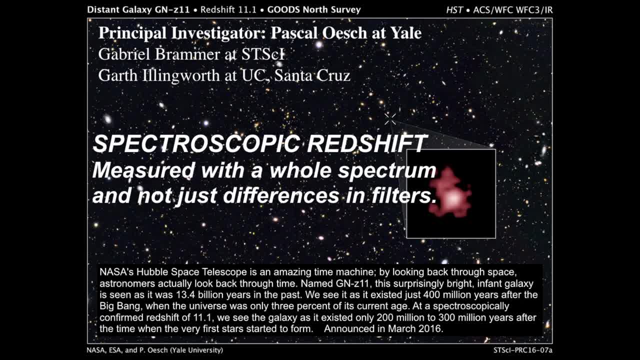 the proof and that we have a pre a some extraordinarily distant objects and there was one that's even that showed a redshift, a supernova in a galaxy inside the hubble deep field. found inside that field some objects that are worth following up on And the Hubble Space. 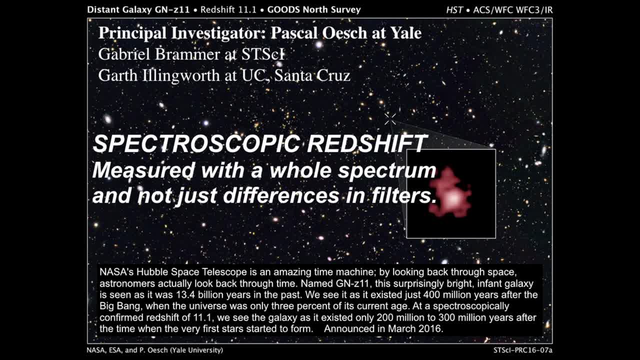 Telescope led by Pascal Osh at Yale in March of 2016,. instead of just doing a photometric redshift, obtained an actual spectroscopic redshift inside of the most distant galaxy. So that is the- this is a much, much more difficult measurement- Photometric redshift. 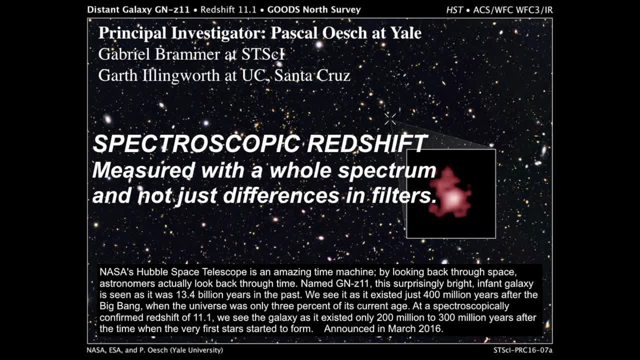 has a lot of problems, but if you can make an actual spectrum of it, then you know that you're actually looking. you can actually determine the spectral characteristics and determine it's actually a galaxy and not a star. So they were able to do this and find. 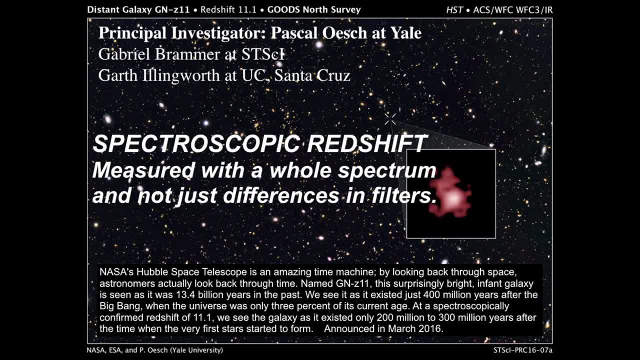 that this was a confirmed redshift by actual spectroscopy, that when the universe we're looking, that the light has traveled to us From this little galaxy for 13.4 billion years and only when they when the couple hundred million years after stars first started to form. So we're almost looking at the very 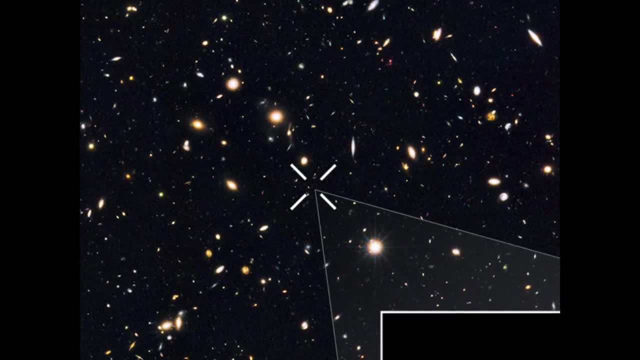 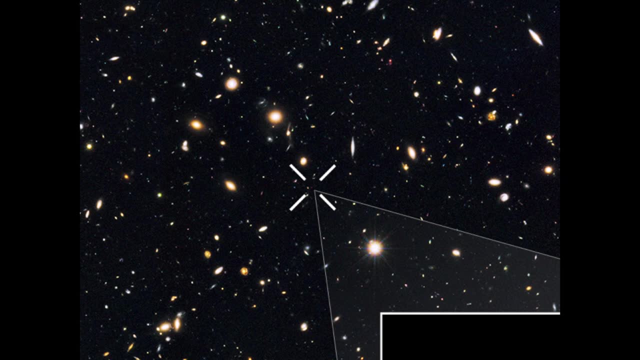 very, very baby pictures of the universe. And so this is an- this is amazing- little discovery, And so you had to really pour over this image to say, Hey, there's a very red like object, Let's take a, let's take a closer look at it. And so here is the image of that. 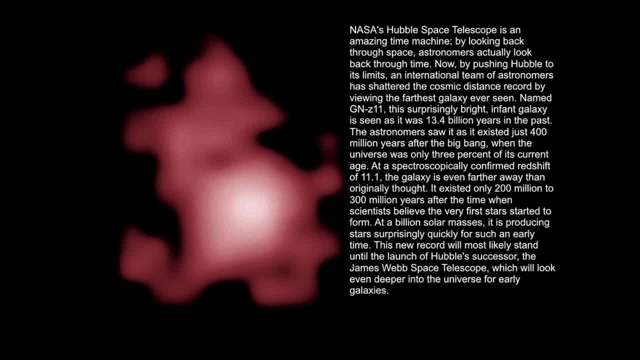 So they cleaned up the Hubble Space Telescope. We saw it from the other thing, that it, that what it actually looks like, And we see this squarey aspect to it which shows we're looking at the actual pixels of the Hubble Space Telescope. 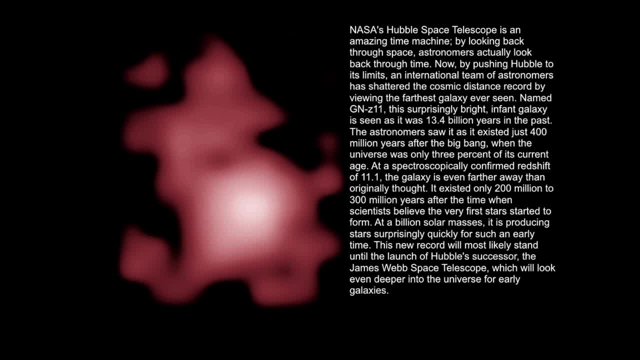 And this is a the shape of this misshapen, really bright galaxy. Well, it was very bright at its time, making huge amounts of blue stars. It now looks red because of the redshift, And so it probably existed the time it existed, about 400 million years after the big bang. 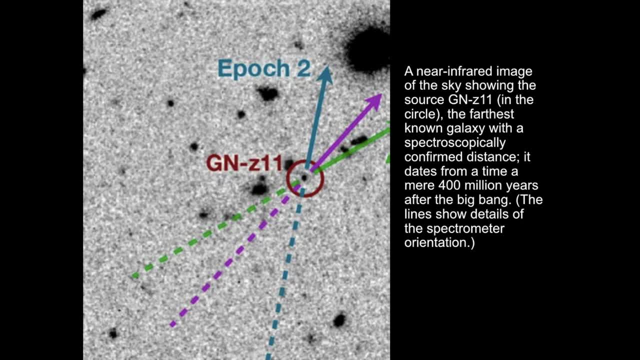 And so how they did this was they took the uh, uh, the spectroscopy, uh, a spectrum of spectroscopic slit of the Hubble Space Telescope and laid it across the object, That's what these lines show- is the location of how the orientation of the spectrometer was. And so 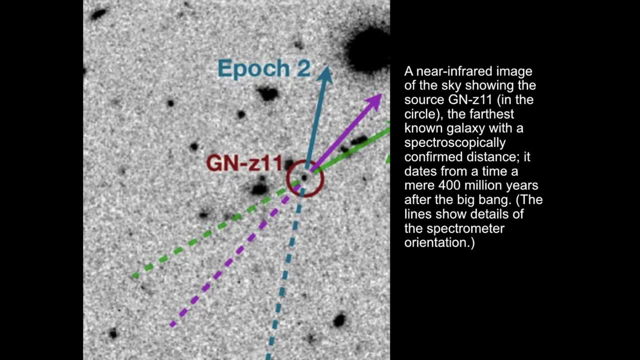 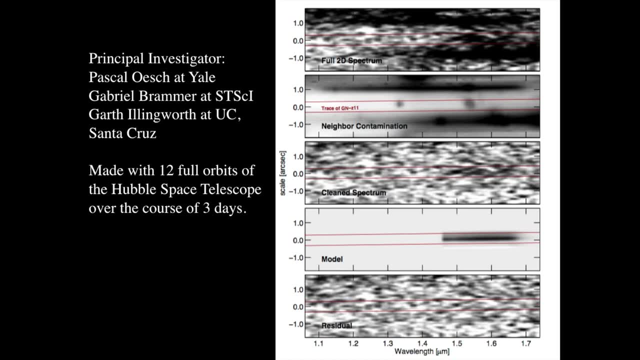 they actually could get some clear space in order to- in order to actually, uh, actually get a, get a view of it. And so what they had to do is they took their full spectrum of it- That's what the top image shows- And then they figured out: well, you know there, 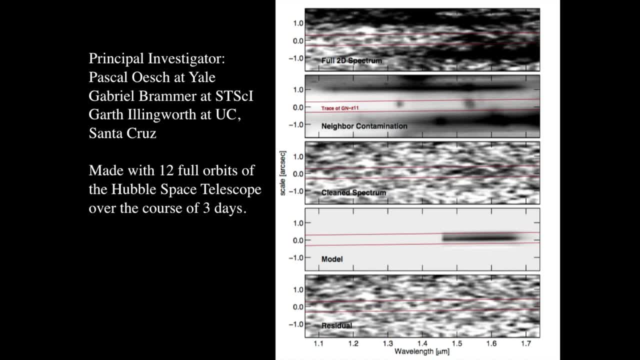 were some bright objects in there so they must be contaminating a little bit. So they reduced the contamination And so what they did was they took a little bit of the bright by the objects there and after they take out the contamination due to neighbors, then they had a. 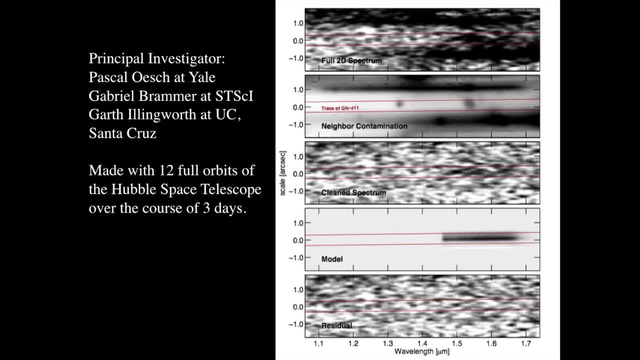 clean spectrum, and then they had a model of what a high redshift galaxy should look like, and then they reduced the clean spectrum by the model and they got what looks like static, and that bottom one is the residual, which is static, and so that's the best you can do, is create static, which is 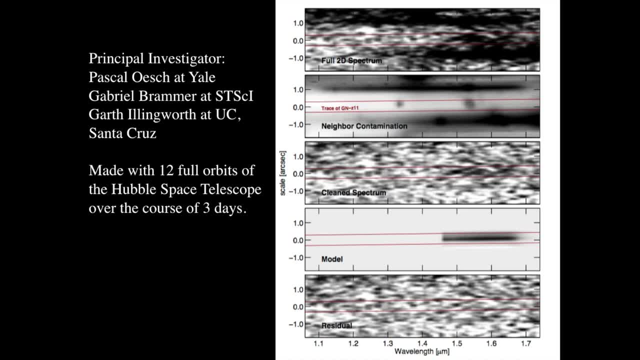 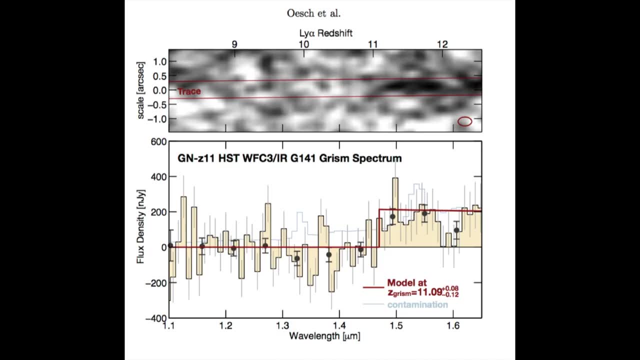 random noise, and so they feel like they've actually gotten it. and so this, since, since this spectrum took 12 orbits and for three days of focusing on this, this one little object, they found that they could model the, the spectrum. so the upper redshift, upper portion is the actual spectrum of it. and 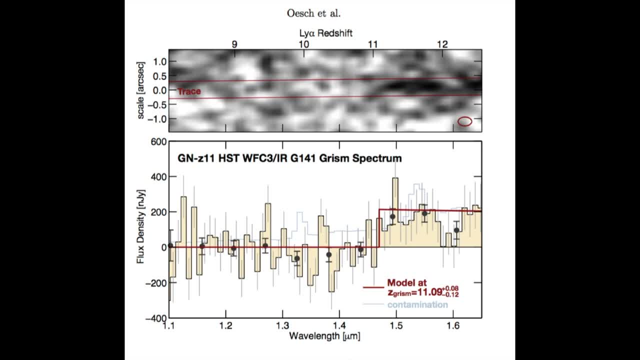 then the modeling uh shows where the data points lied and how they could actually say, okay, it's basically noise to the left. and then they have an actual spectrum that begins with the, the, the grism, showing it's an 11.1 uh resin redshift object. 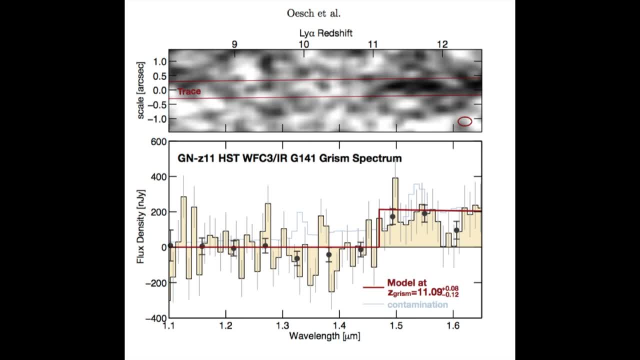 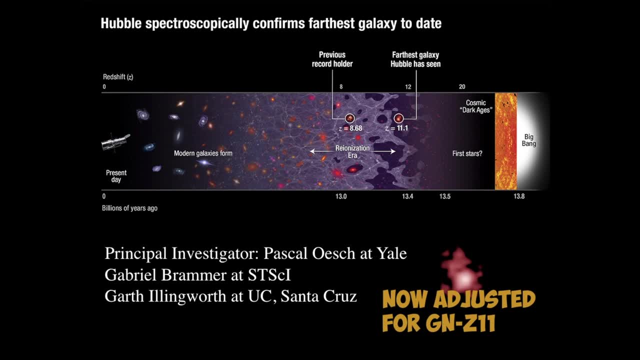 so this was, uh, the is. it is currently the highest redshift object measured spectroscopically, which is really interesting, so it's the farthest galaxy that hubble probably will be able to see, and it still doesn't get to when stars turned on. it's looking at extraordinarily deep objects, but 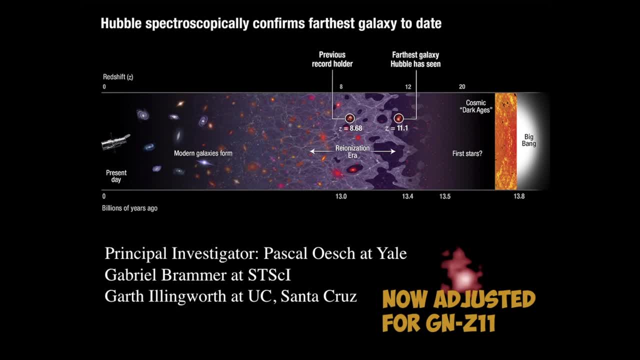 hubble's. but hubble's uh aperture is not large enough. it simply is not a large enough aperture and it doesn't have the infrared capability. and that's going to happen in the future, so it's going to have to wait till the james webb space telescope is launched. so the object, the previous, 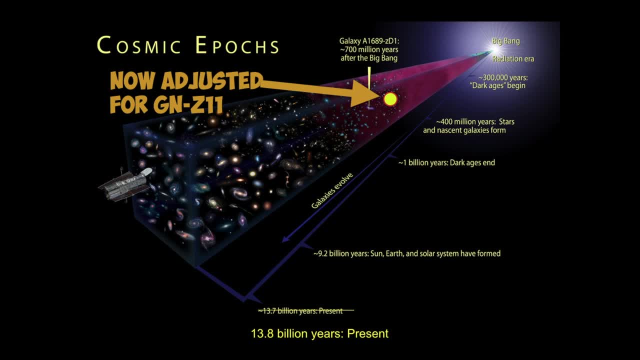 record holder was about 700 million years after the big bang. now it's something that's looking at about 400 million years after the big bang, just after stars started forming- only 200 million years. so we could think that if stars that are super massive take only a 5 to 10 million years to, 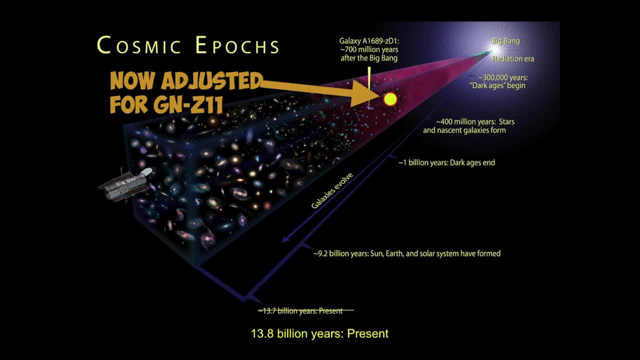 actually form, then potentially we're looking at the first four or five or six generations of stars being formed in that little, in that misshapen structure, and they don't actually look like they're going to get to us in time- sort of weird galaxy And hopefully the James Webb Space Telescope will be able to see. 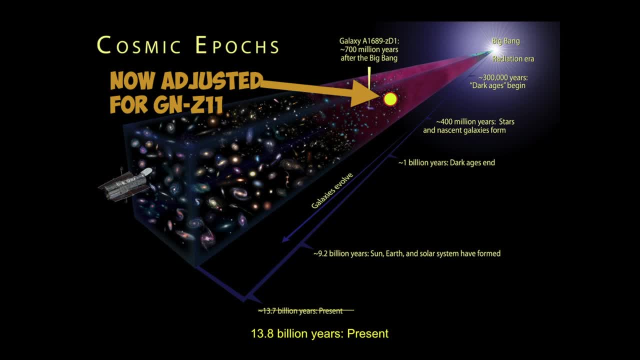 things, And this diagram kind of shows us. what we've been seeing is that structure forms with time, And galaxies evolve from being small, misshapen, tiny, bright things and they merge and collide into larger and larger and larger objects until they form. 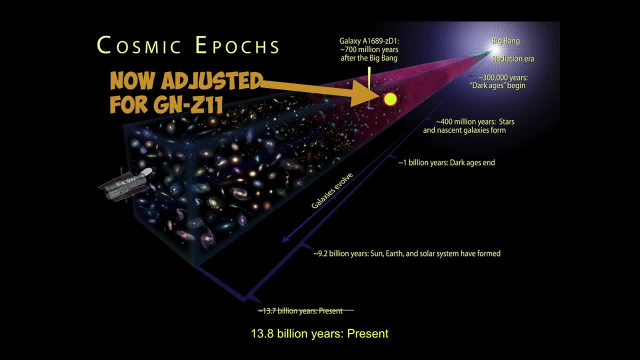 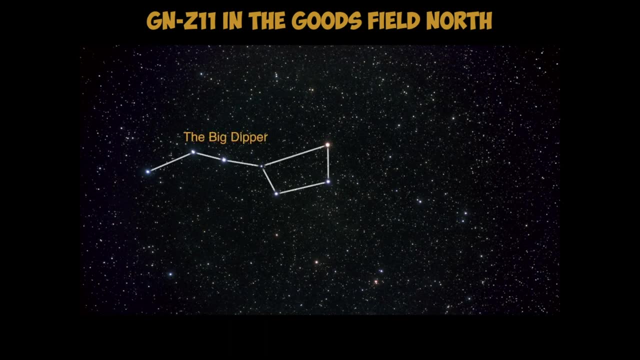 either supermassive ellipticals or small ellipticals, or grand spiral galaxies. So just to give you a feel for where this location is, where that tiny, tiny, tiny galaxy is, we're looking at Ursa Major, the Big Dipper in the sky. 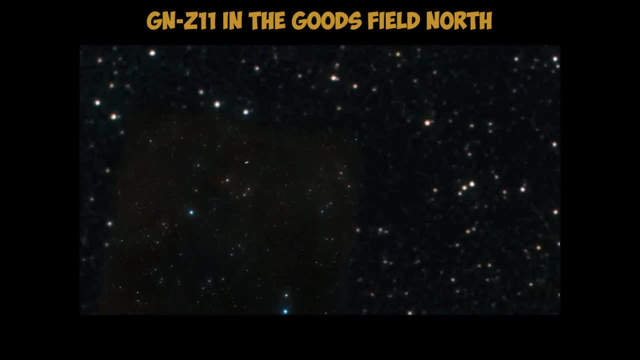 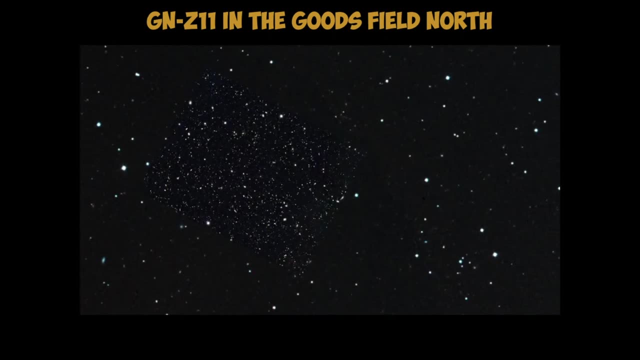 and so let's zoom in to see how tiny a patch of sky that really is that we're looking at. And we keep zooming in and zooming in and falling into this tiny patch, into the Goodsfield North Survey, All the way into tinier, tiny locations. 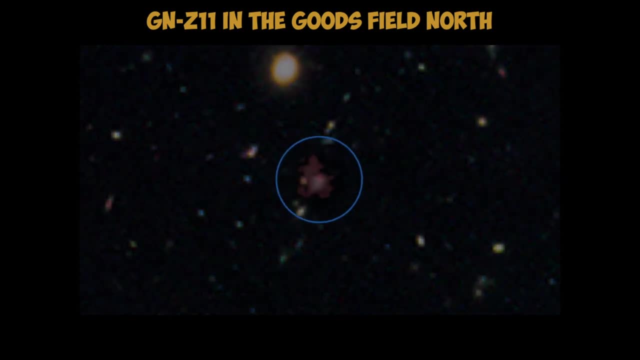 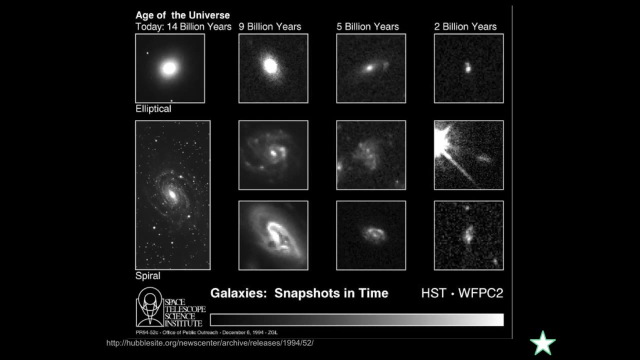 and there it is, one little bitty object seen in observed spectroscopic galaxy by Hubble. And yeah, it's right off the handle of the Big Dipper. So what we've learned by looking at these deep, deep, deep surveys, which we'll call pencil beam surveys, 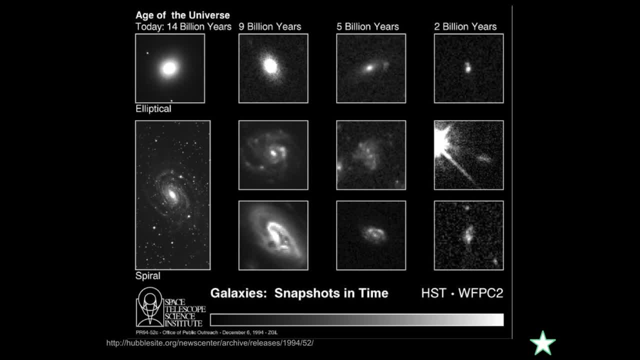 like the Hubble Deep Field, Hubble Ultra Deep Field, Extreme Deep Field is that we're able to see galaxies in different states of evolution, And so we can think of what a spiral galaxy like our Milky Way would look like when the universe was only 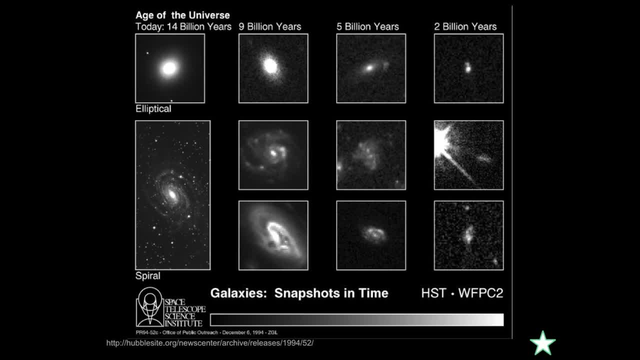 2 billion years old. This is what the far right hand pictures might see And as time progresses, from, say, right to left. I wish it was the other way, but hey, we're going this way. So when the universe is only 2 billion years old, on the far right, 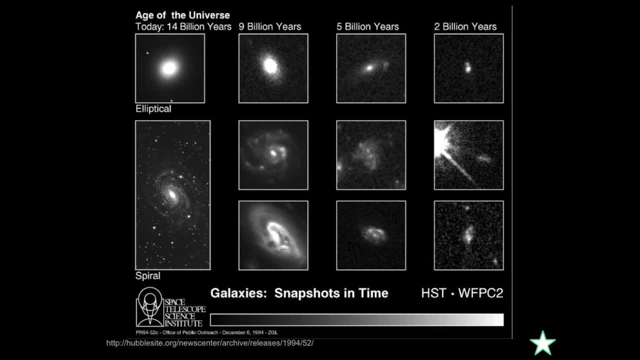 things were tiny, bright and misshapen And, as at 5 billion years after the Big Bang, we see multiple cores and multiple interactions in some bright areas, but not uniformly bright across the object, but they're larger and there's some structure that's appearing By 9 billion years. 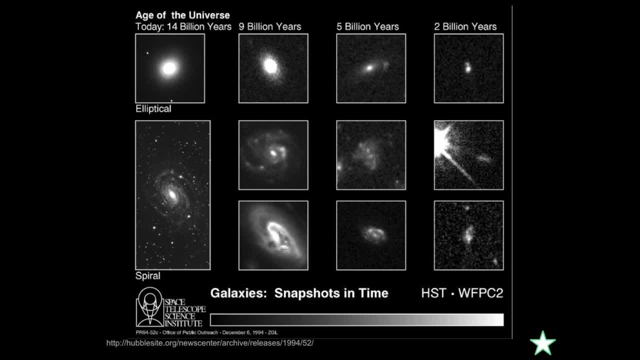 after the Big Bang, we're able to see things that are not necessarily visible to the naked eye. objects have gotten much more complex and larger in scope and by the today type time, 13.7 billion years later, we're rounding to 14, just because because this was in 1994, and so their dark energy. 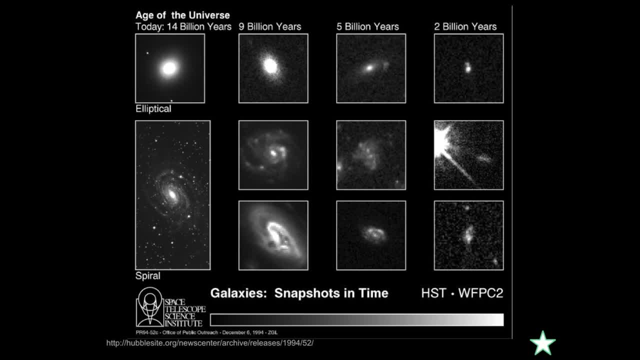 still had not been really discovered yet. so here we go, but 14 billion years, 13.7 billion years later. i should really adjust the slide. we see spirals and giant elliptical type objects, so galaxies evolve with time. we do not see milky ways in the deep past, so therefore,